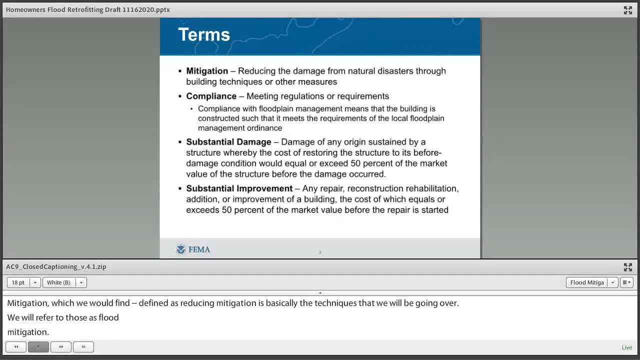 refer to compliance with floodplain management regulation, which means that the building is constructed such that it meets the regulations. If we were trying to reduce risk from high winds, we would refer to that as wind mitigation Compliance. that's, meeting the regulations, or 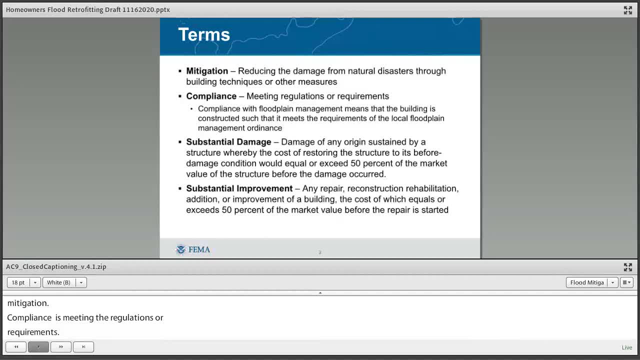 requirements of the local floodplain management ordinance For buildings that are located within the Special Flood Hazard Area or just commonly the flood plain, we would consider substantial damage. Substantial damage is damage of any origin. That means, whether it's flood damage or high wind damage, or both, fire any origin sustained by a structure whereby the cost of restoring the floodplain is limited. Most of the damage is received for that particular project. Most of the damage is received for that project. Most of the damage is received for that project. Most of the damage is received by professional flood site management, local flood. 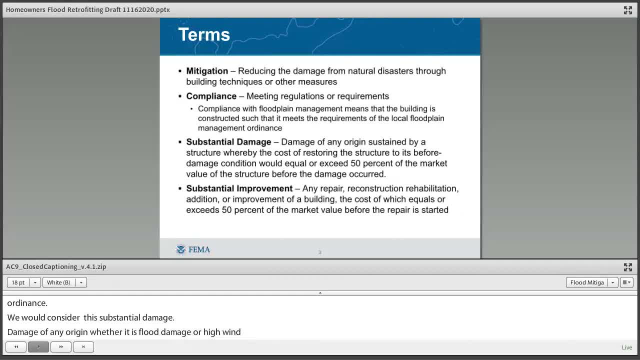 land management, water, rail water, water, storm water, weed, fire and other specific types of problems. structure to its before damage condition would equal or exceed 50% of the market value of the structure before the damage occurred. This is a key consideration. 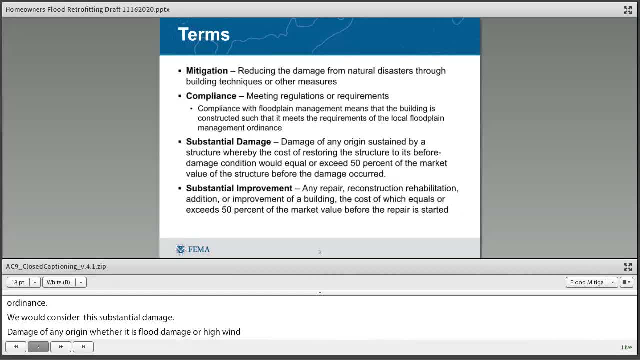 when you're looking at a building and trying to decide whether the building needs to be brought into compliance or whether the building is fine as it is. So that that's going to be a key term that you're going to have to look at Also. 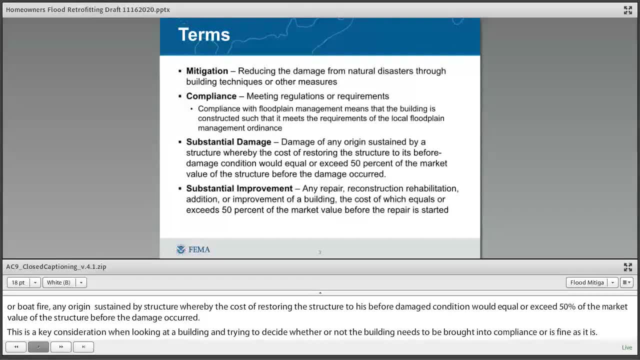 connected with substantial damage is another term. This again only applies to buildings that are within the special flood hazard area or the floodplain. Substantial improvement: Any repair, reconstruction, rehabilitation, addition or improvement of the building, the cost of which equals or exceeds 50% of the. 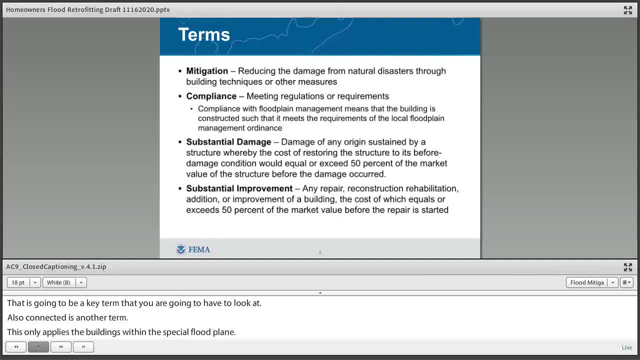 market value before the repair is started. Now, if you have a building that was damaged during this event and you are looking at doing repairs to the building and you're looking at maybe some other improvements, then these two factors would be combined and you would look at what we would refer to as the 50% rule, for that overall, We often consider those repairs from substantial damage to be considered within substantial improvement. So this is a key consideration for you as you as you kind of look at what projects you're you're looking at and what repairs you've done. 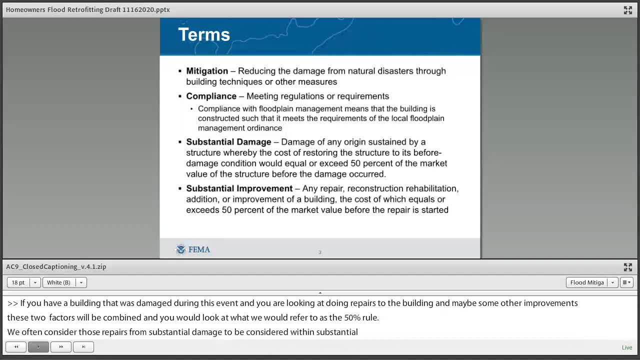 Now you do need to work, if you're close to this, with your local floodplain administrator to see how they are counting these substantial damage and substantial improvement requirements. Sometimes it's per year, sometimes it's over a period of years and sometimes it's over the life of the building. So 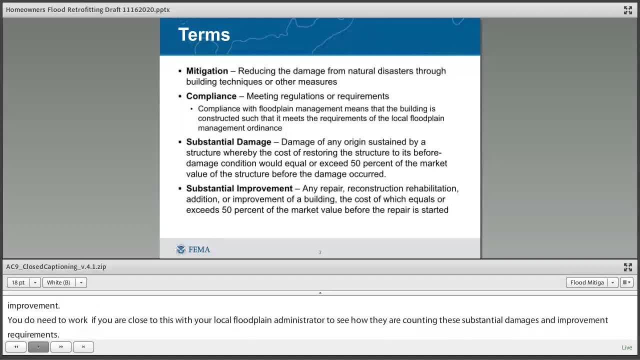 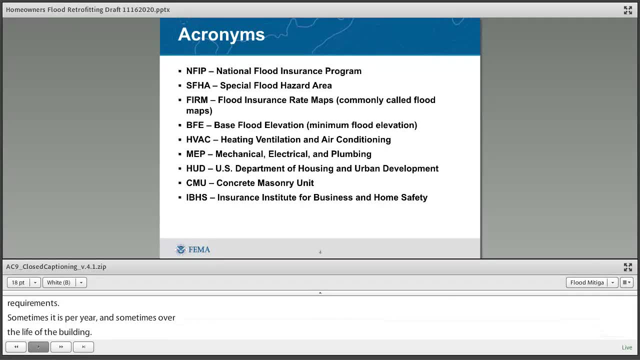 this would be helpful for you to go and contact your local floodplain administrator in order to find this out. Now, some acronyms that will be mentioned throughout this NFIP, that's, the National Flood Insurance Program, which includes both the insurance program as well as the overall program requirements that we'll be. 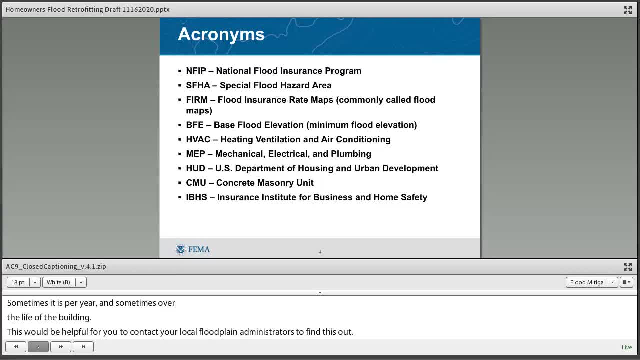 talking about today- SFHA- Special Flood Hazard Area- or the floodplain that you may commonly refer to it as FIRM. this is a flood insurance rate map, or the flood maps BFE- the base flood elevation. This is often the minimum flood elevation that is shown on. 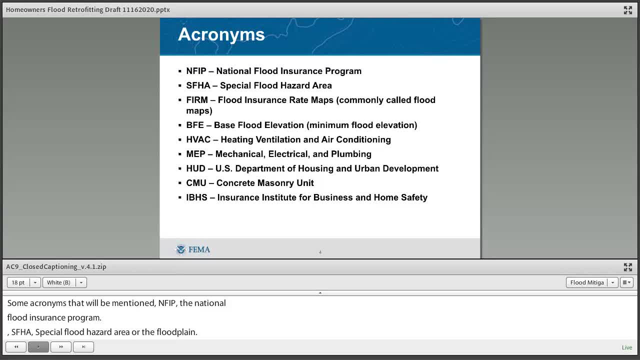 the flood maps. Your community may have additional requirements to build, say one foot or two foot above the freeboard requirement, and that may be your community's local minimum requirements. Some of the other terms that you'll hear me use: HVAC, heating, ventilation and air conditioning, MEP- mechanical, electrical- 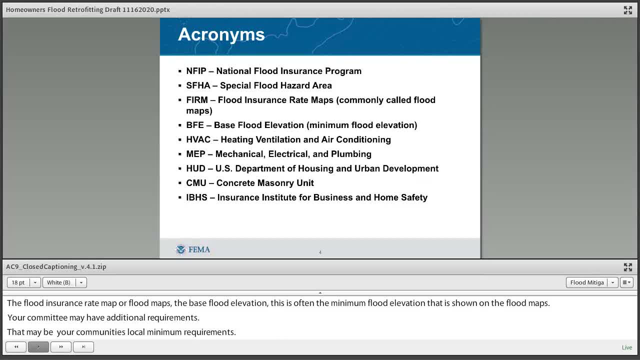 plumbing system. This is all sort of your normal building systems that we would have in a home, And then we'll refer to HUD, housing and urban development, CMU, concrete masonry unit. That's basically a cinder block, in common terms- And then we'll have a reference at the very end to IBHS. Now they've 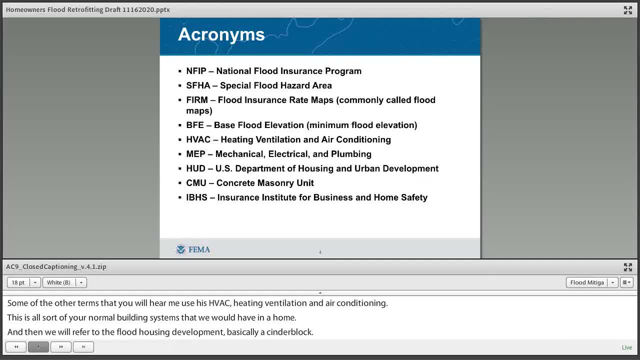 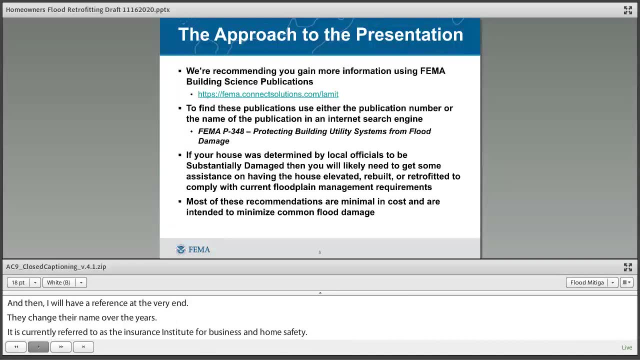 changed their name over the years. It's currently referred to as the Insurance Institute for Business and Home Safety, but it was originally the Institute for Business and Home Safety, which is where they got IBHS from. The approach to the presentation, We're going to give you some ideas on doing mitigation, but ultimately we'd prefer that. 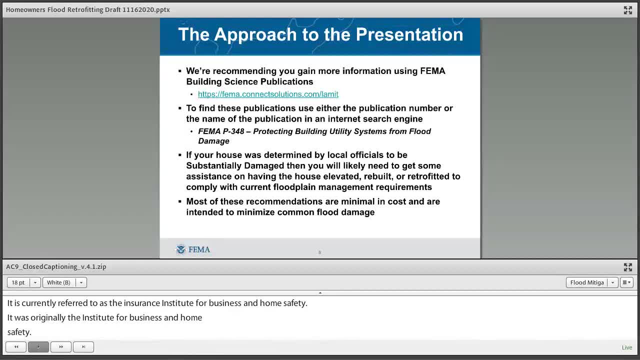 you gain most of the information using FEMA building science publications And there's a link here for you to get those FEMA building science publications. The best way to find these publications is often to use an internet search engine. So to find these publications, either use the publication number or the publication name. 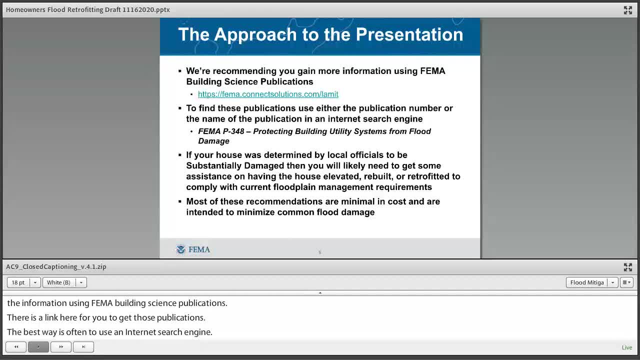 in an internet search engine to find the publication And that should bring up a link and that will either bring you to the FEMA webpage or possibly directly to the PDF file. So, for instance, with this publication, if you typed in FEMA P-348, you would probably find the file, Or 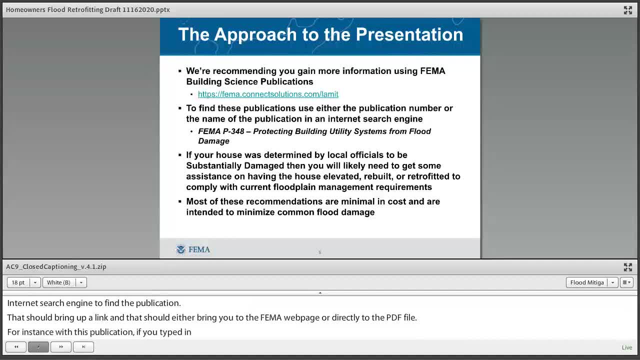 if you typed in protecting building utility systems from flood damage, you would also. you would also be able to get this link Now. you don't need to type in often the publication number and the name. It's usually one or the other that will bring it up in. 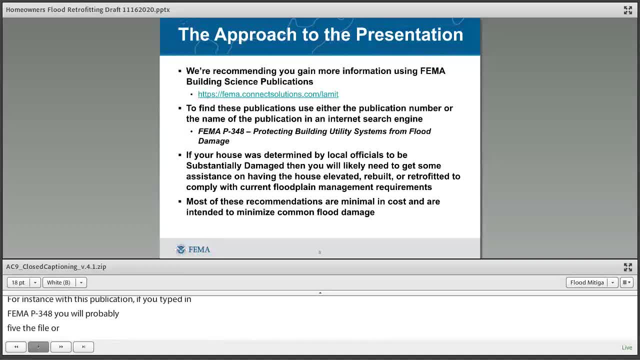 most search engines. If your house was determined by local officials to be substantially damaged, which we just discussed, then you will likely need to get some assistance on having the house elevated, rebuilt or retrofitted to comply with the current floodplain management. 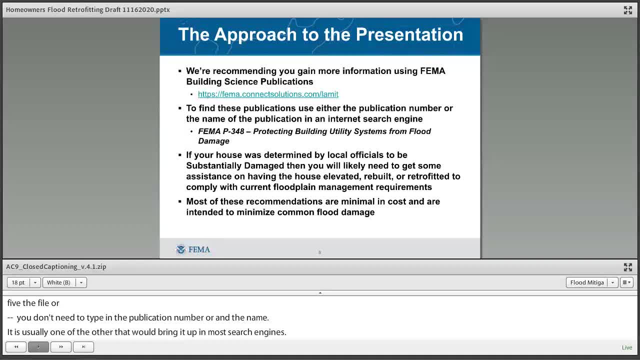 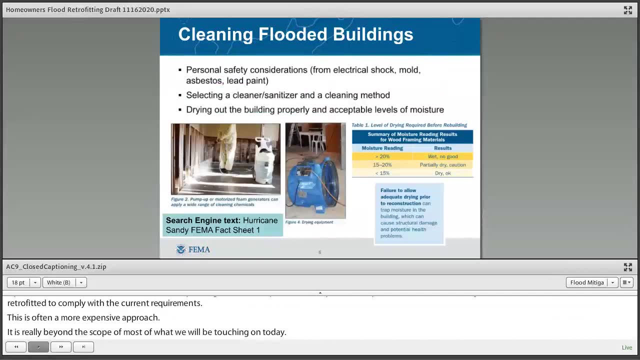 requirements. This is often a more expensive approach and really beyond the scope of most of what we're going to be touching on today. Most of the recommendations that we're going to be covering are minimal in cost and intended to just minimize common flood damage. So the first 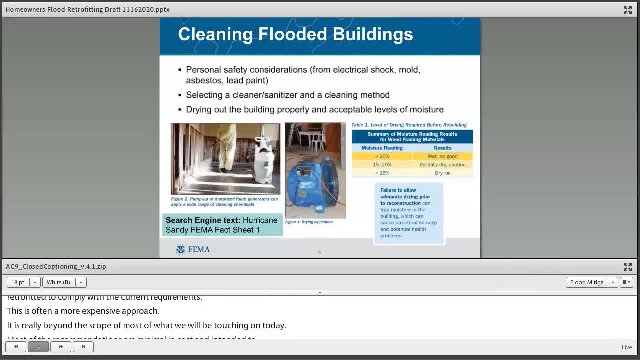 thing we'd like to talk about is obviously just getting the building dried out, And you'll see that we refer to a fact sheet: 001, 002, 003, 004, Hurricane Sandy: Fact Sheet 1.. Now, throughout this presentation, you're going to see a lot. 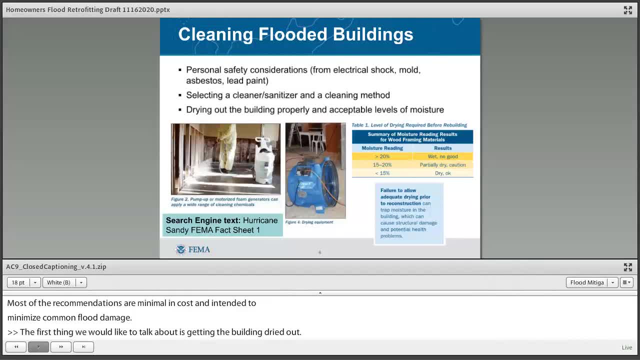 of references to Hurricane Sandy fact sheets or fact sheets that were developed for some Iowa floods or Hurricane Isaac fact sheets. These fact sheets may be older. However, there is a lot of consistency throughout the nation and throughout past storms that are going to be really helpful for you to understand. 001, 003, 004. 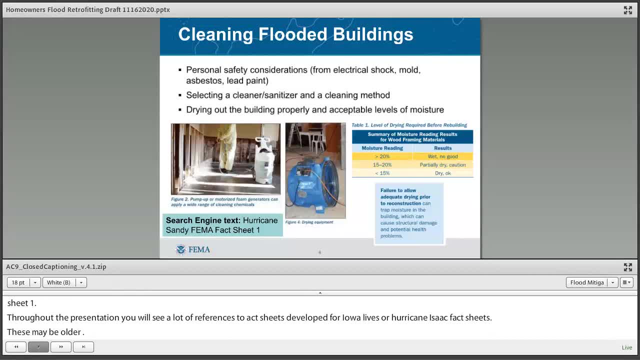 Hurricane Sandy Fact Sheet 2.. So you'll hear us talk about what's a good thing to do, and we're never going to be putting a lot of emphasis on what you need to keep out and having a lot of fun with the future of your property. 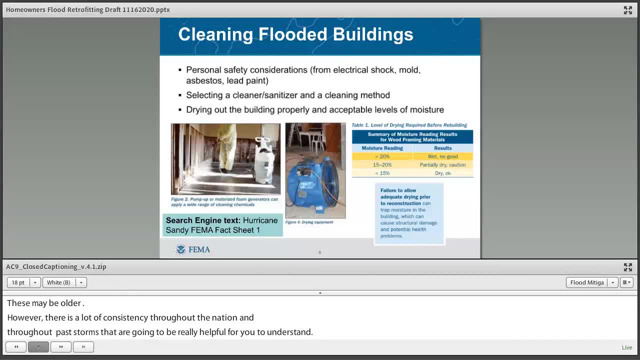 001, 003, 004, 005, 006, 007, 008, 009, 0011, 0011, 0012, 0012, 0013, 0014, 0015, 0016, 0017, 0018, 0019, 0020. 0022, 0023, 0024, 0025, 0026, 0027, 0026, 0028, 0029, 0030, 0031, 0034, 0035, 0045, 0046, 0048, 0057. 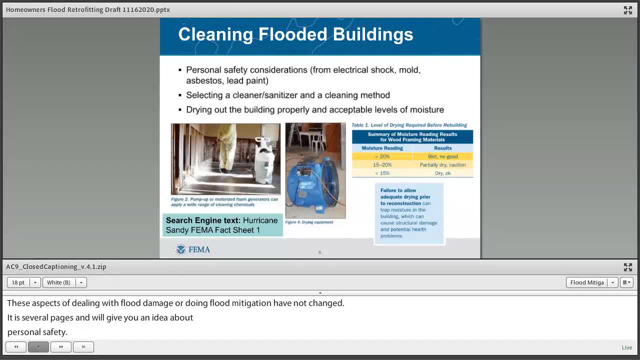 0059, 0059, 0050, 0060, 0050 01, 0050 01- 0050 01. asbestos and lead paint are going to be more common on older buildings and it's important that you get some of these materials tested to make sure that. 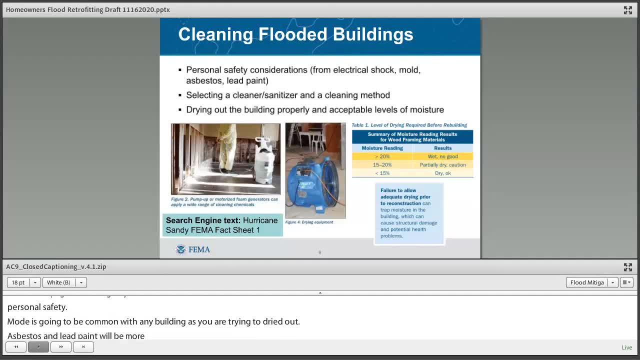 you're not going to expose yourself, selecting a cleaner and sanitizer and a cleaning method. there's a lot of things in floodwater that may be dangerous and it's important to clean those out, as well as addressing this mold issue that we've discussed and finally drawing out the building properly and reaching 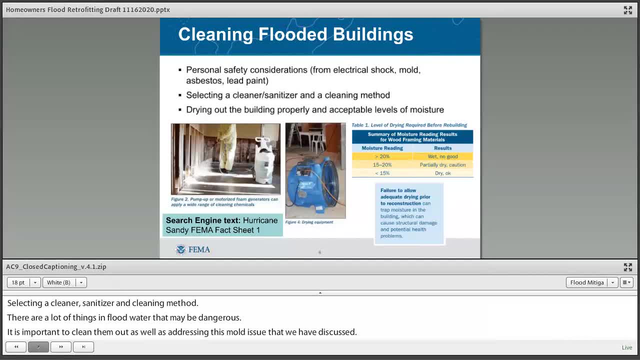 acceptable levels of moisture. so you'll see there's a little table on some accessible levels of moisture. the main point with this is that we don't want you to cover up walls in terms of putting, maybe, drywall and insulation back in a wet wall or putting a floor covering over a floor. 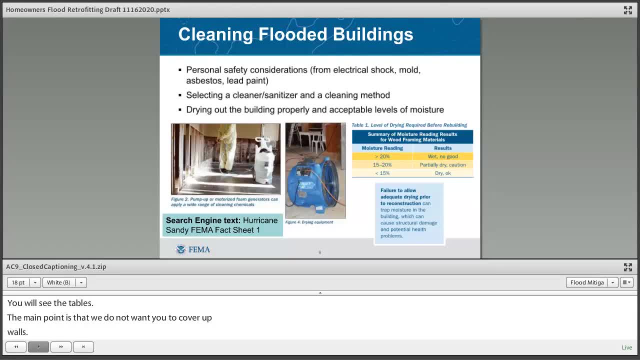 ceiling and then putting a single floor out into the floor. so that's an example of putting a floor covering over a floor set or a floor set or a floor cover, and that's that's not completely dried out. what can happen is that you can still have mold growing underneath the floor system or within the walls and and that 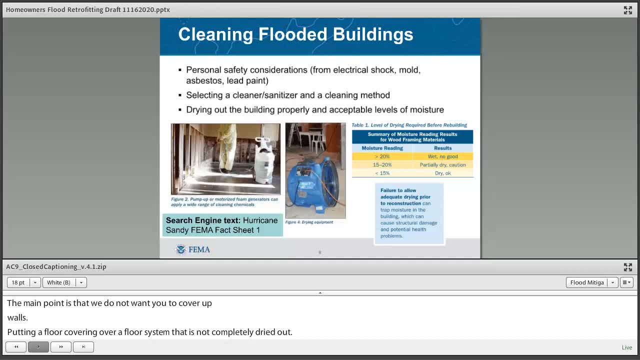 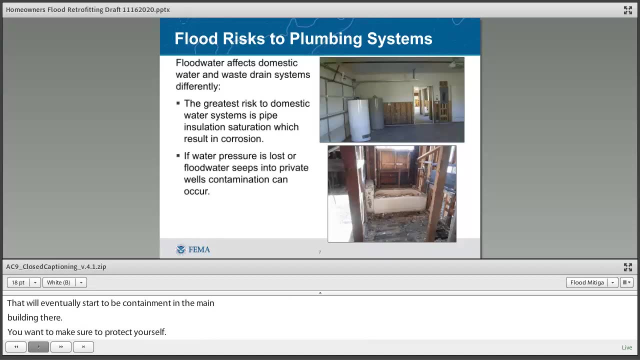 will eventually start to be a contaminant in the main building air. so you want to make sure to protect yourself against that, and that's why we really try and discuss how to properly dry out the building. so we're going to be talking about these building systems now. flood risk to plumbing systems is. 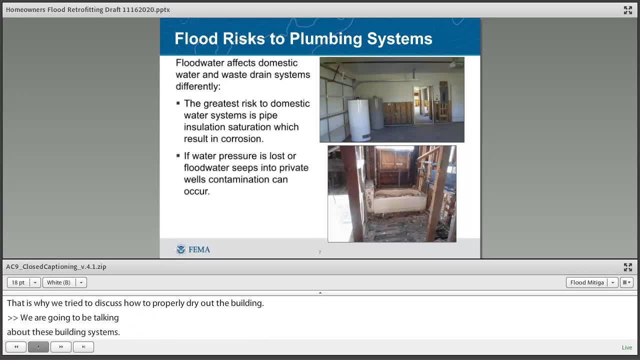 the first item that we're going to touch on. flood water affects both the domestic water system- so the water coming into the building- and waste drain systems differently. the main risk to your domestic water system is water- that that flood water that comes in it saturates the pipe. 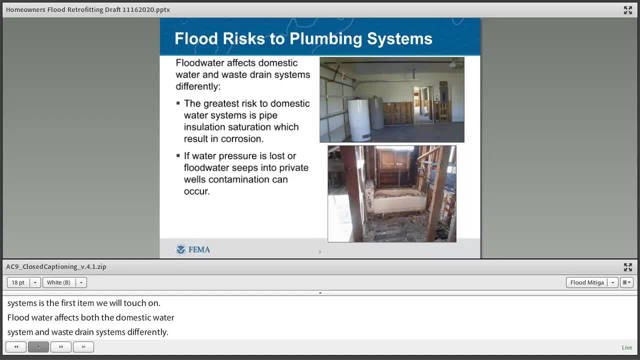 or the insulation around the pipe and for the metal fittings that can cause corrosion, and said we want to make sure that we're not having problems with damage fittings that could be leaking water later on. the other thing that we can- we will see some times- is that if water pressure in the system is lost, 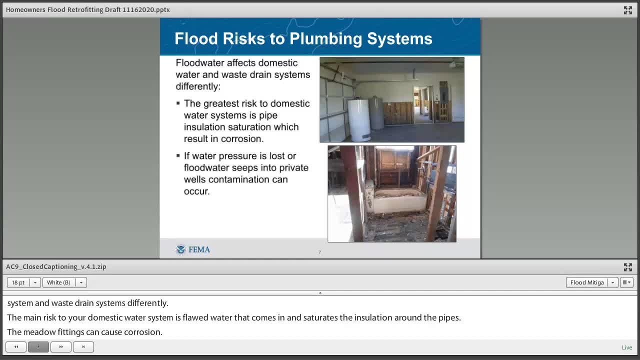 that can seep into your water pipes as well as private wells, and cause so. we want to make sure that we're protecting ourselves against the potential for water to seep in and making sure that we've sanitized the water lines properly in order to protect you later on from consuming. 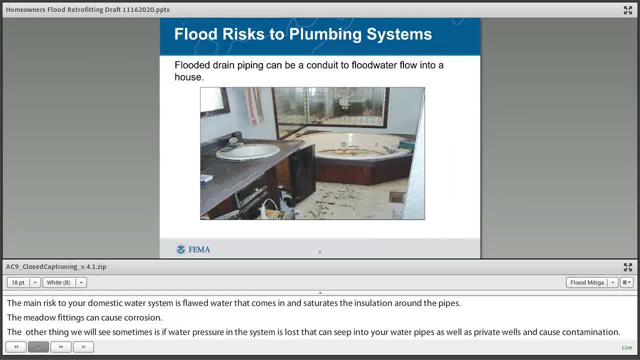 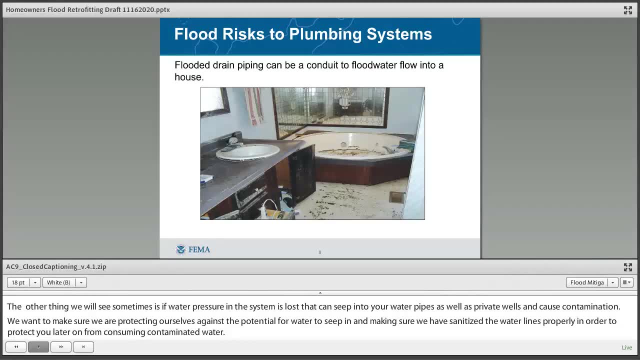 contaminated water In terms of the drain lines. drain lines can be a way for that flood water to get inside the house and and what we see is basically the backflow of those flood water and sewage into the house. and you'll see this picture that we have where sewage is backed up into the house and it is. 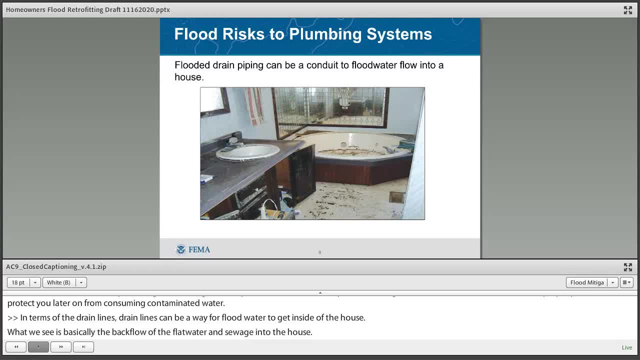 covered this whole bathroom area as well as other parts of the house, and you'll see that it ruined the cabinets, ruined a bunch of the wall systems, the floor systems and that sort of thing, And we'll talk about how to protect or mitigate against these types of issues. 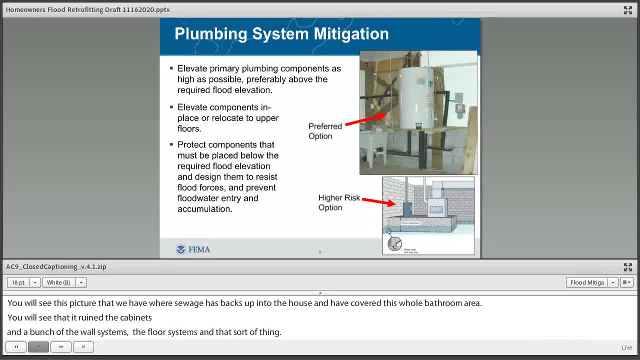 using backflow valves, So most of the plumbing systems. we recommend that you consider elevating those components as high as possible. Now, that could be relocating these components to a higher floor or elevating those in place. If you're a low-income person, then you can use a water heater. Now the picture that 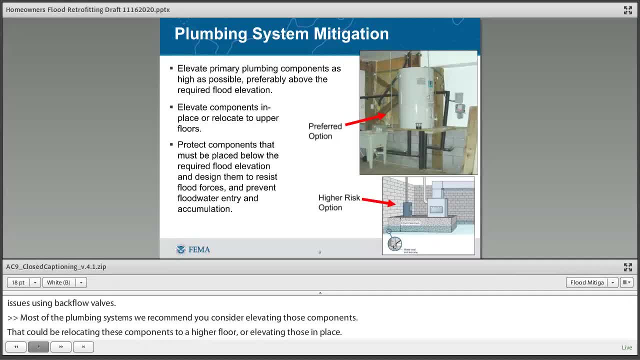 you see on the upper right shows a picture of a water heater that was elevated in place. A lot of people have their water heaters located in garage areas and often those are not terribly high off the ground and this means it can easily be reached by flood waters that get inside that area and then it 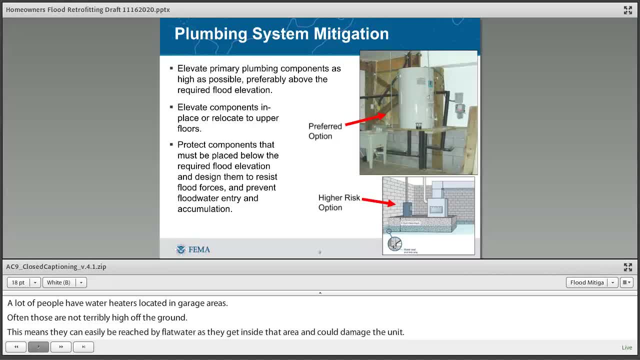 can damage the unit. So if we could look at elevating those units up off the ground, we can provide a lot of water into the house, lot of protection, before the floodwaters actually reach those units. The other consideration is actually looking at bringing that water heater either into the attic. 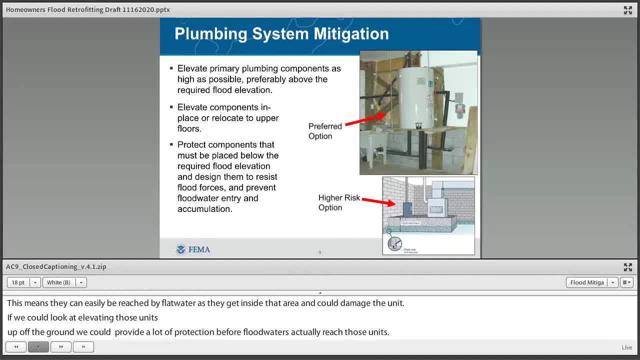 area, which is common in some homes, or into the living space. Or the other option is: maybe you've got a water heater like the one shown, or a tank water heater and you may be looking at a tankless water heater from the space. Now there are. 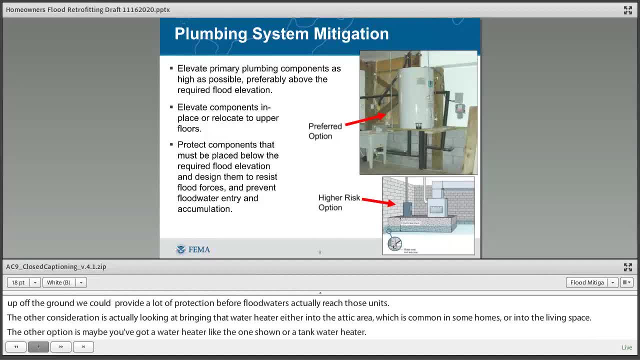 trade-offs to looking at tankless water heaters, and I would encourage you to look at those trade-offs over time and make sure that that's a good option for you before you consider switching. But those are just different ways that you might be able to still not lose too much. 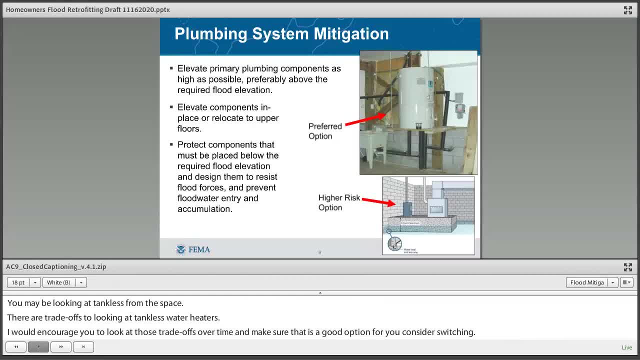 space inside the home and move the water heater inside the house. Now, if you move it inside the house or inside the attic, draining or having a way, in case there's a leak in the water heater, to drain, it is really important. So that's another consideration that you have. 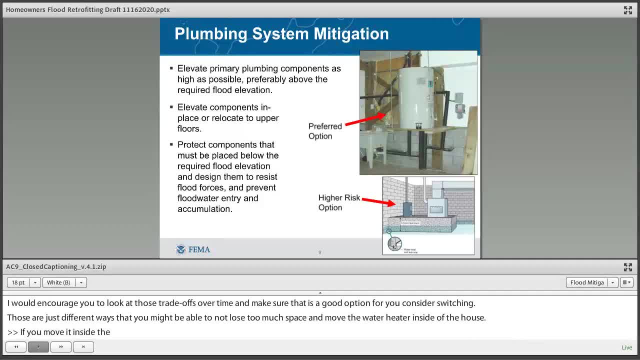 But these are the recommended methods, either, like I said, in place or in upper floors. The other option that you have, if you can not move those, is protecting those units in place. The lower right picture has a water heater that's placed on probably a small pedestal just. 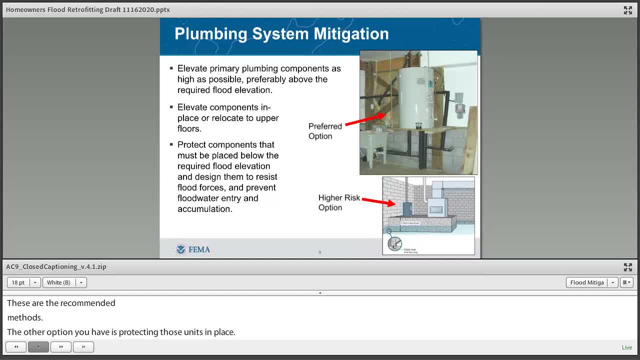 above the ground and a heating unit side by side. this is common for homes and in this instance they couldn't relocate it, so they built a little wall system around that. now the problem with that wall system is that once that wall system gets over topped, you can end up with the same amount of flood damage. 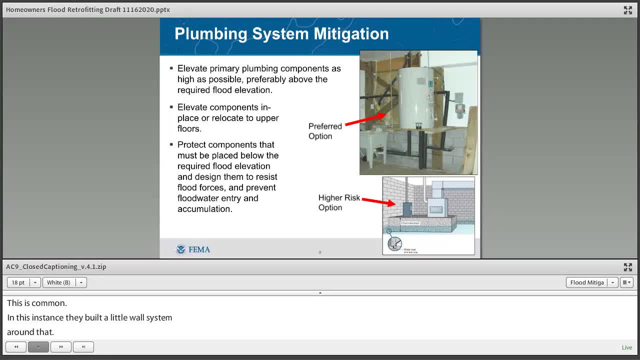 that you would have had had you not had the wall in place. the other consideration, once you do wall systems, is making sure that there's clearance around that wall system so that you can do maintenance, that somebody can get in and out, that they can check the unit, that they can maintain the unit and that 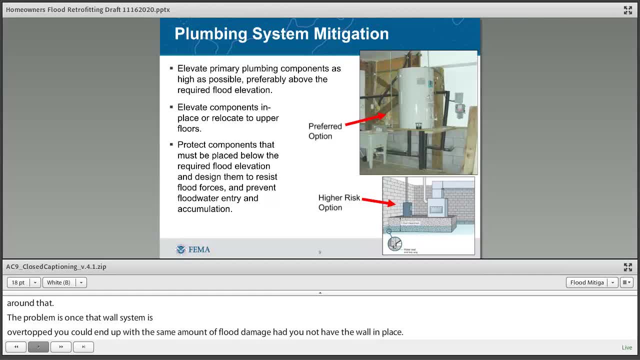 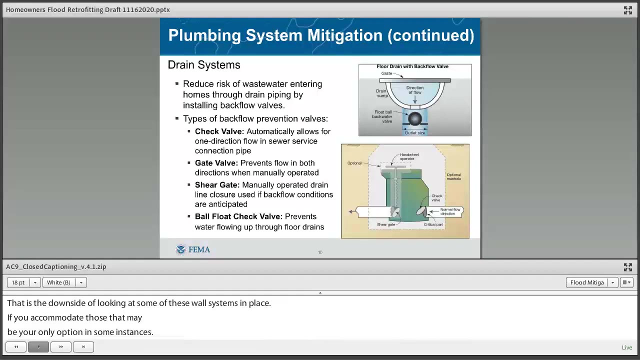 there's proper ventilation around some of these units. so that's the downside of looking at some of these wall systems in place, but if you accommodate those, then that may be your- your only option in some instances. so we wanted to provide that. if we look at drain systems, so moving over to the water from that, the drain systems back. 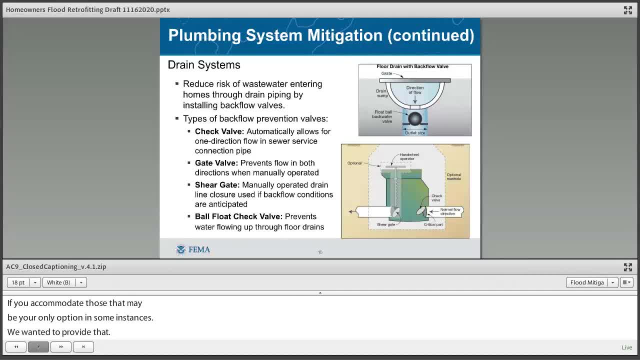 flowing into the house. we recommend you consider a backflow valve. there's a few different kinds of backflow valve protection. mainly we would categorize those into either a, an automatic or a manual valve. backflow valve and the automatic backflow valve is a great option for people that that may not have the ability to open up. 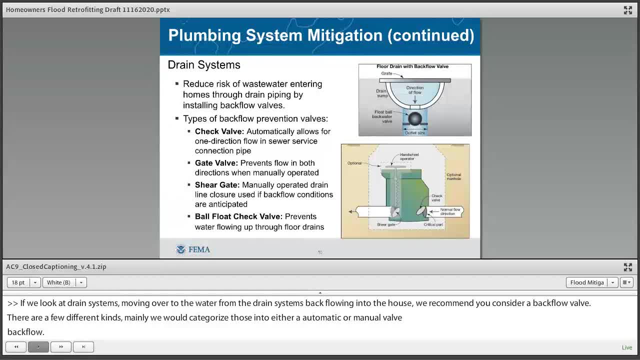 go outside to open up a cover, shut the valve, or maybe they aren't at the home all the time, and so an automatic backflow valve may be a really good option for those people. the more reliable option is usually the mechanical or or manual backflow valve. 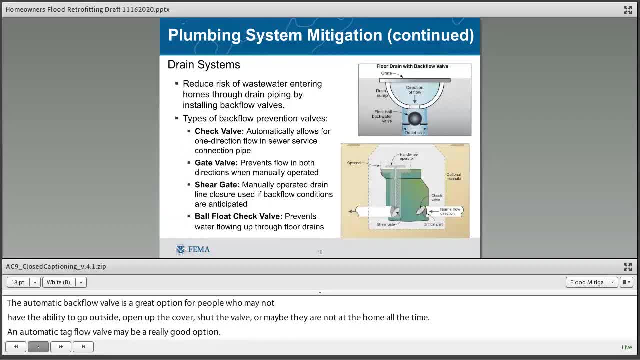 where you go outside you remove a little cover, you close the valve by hand and then shut the cover and those are probably more reliable. but again, you do have to actively do that before you can can get it closed. but both of these are covered and we'll kind of talk about where they're covered, scared in terms of Alsha supply ds with an automatic backflow valve, live water Granate hopeless is peeled out. that an discomfort and those are covered and we'll kind of talk about where they're covered and turn to the in terms of where that he may or may not have the operatingvant or most of these zones. we're not easier to RCA and energy companies and umbrellas will walk instead of the ref. Heidi, when you need replacing the Richeland in several other things so that Y estamos体 to learn mostly about�. 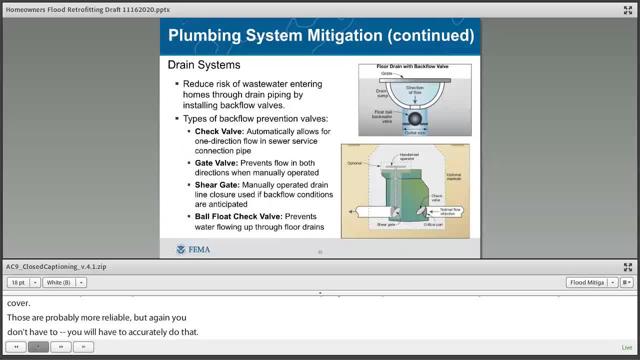 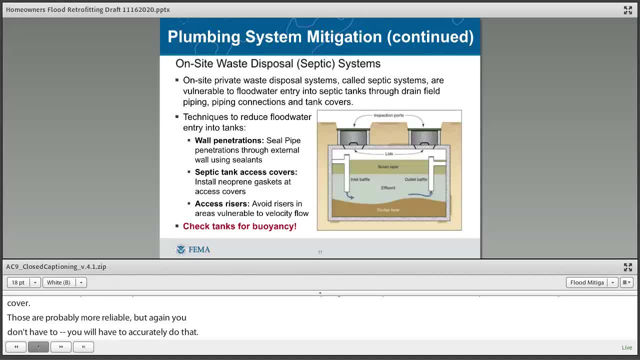 in terms of some more description on them in a minute, when we talk about the FEMA publications. The other consideration in terms of plumbing systems is if you have on-site waste disposal or a septic system. this is another area where we have cause for concerns. 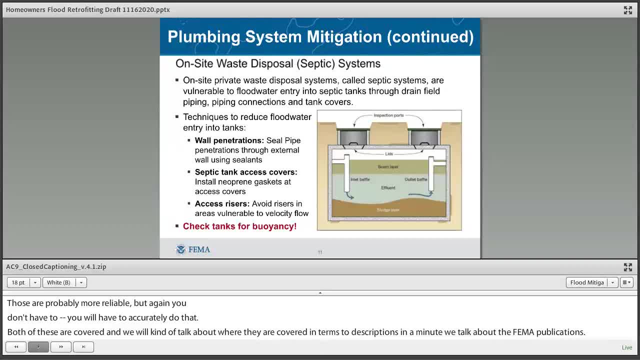 and floodwaters can either get in the inspection ports- You'll see those in the diagram, at the very top of the diagram- and water can get into those if they're not properly sealed. The other thing that we see water coming in, they usually back up from the septic field. 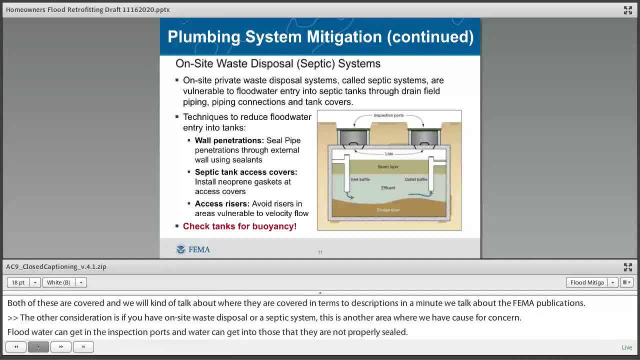 which is the next portion of a septic tank that moves out, that the floodwaters can kind of move back, flood the septic tank and then go back the other direction, And this is where a backflow valve would be very valuable for you to keep it from coming in. 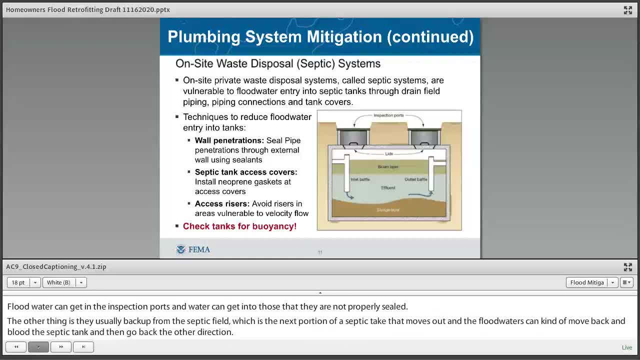 But the other consideration that we have is is that with a septic tank there's usually an air gap at the very top of the septic tank. If you get the soil around the septic tank saturated, then you can end up with buoyancy or floating issues. 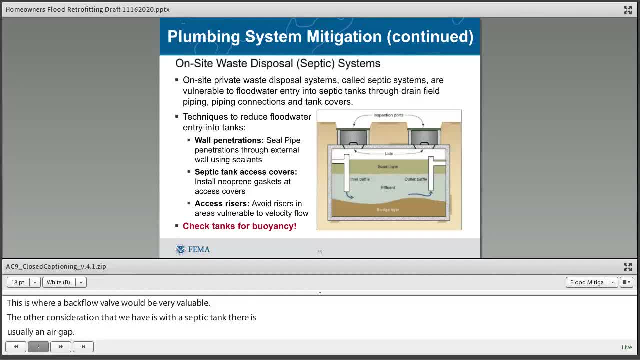 that basically, there's more water on the outside and so you have an air gap or a lot of air gaps potentially inside that septic tank and it can cause it to float. So we do want to make sure that you have that in mind. 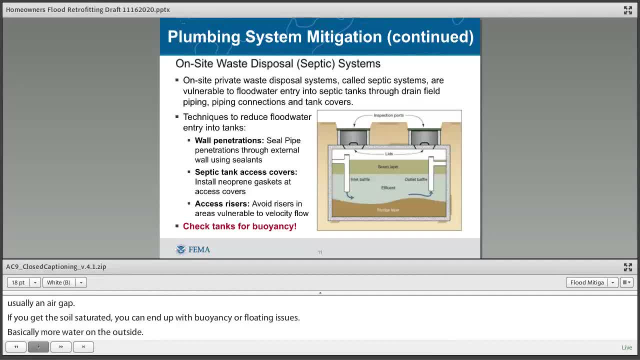 Make sure that the septic tanks are anchored properly so that they don't float, because not only is that going to damage that actual septic tank, but also the pipes running from your house to the septic tank. it will damage those, as well as the pipes going out to your septic field. 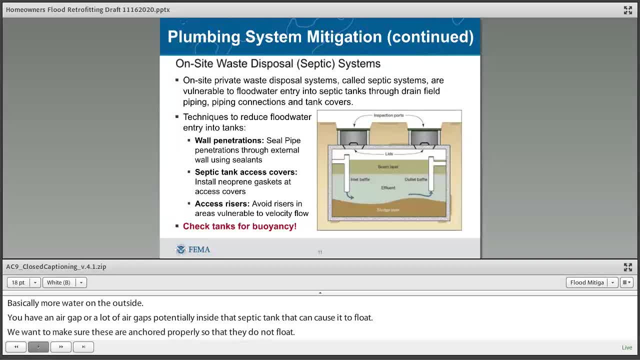 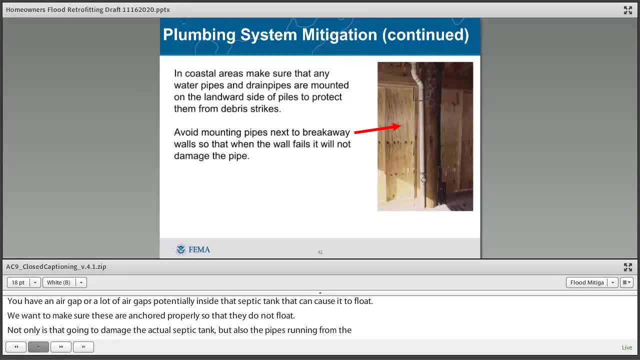 So there's a lot of damage that can happen if you don't have a properly anchored septic tank. Another consideration that you'll want to look at is if you were in a coastal area and you were talking about a house that's on an elevated foundation. 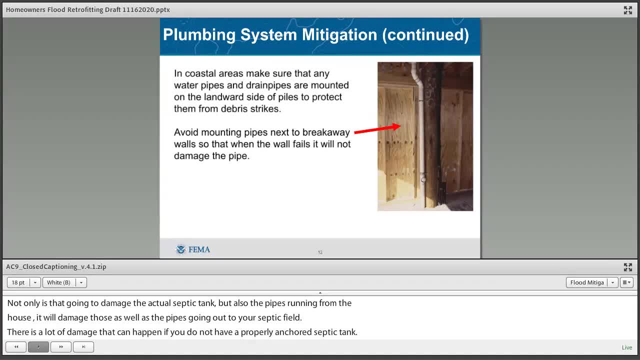 so piles columns in those instances. a lot of times, people have what we would call breakaway walls. Now, a breakaway wall is a wall system that is intended to fail under the flood load. The reason why we want these breakaway walls to fail is that these walls breaking away can relieve the stress on the foundation. 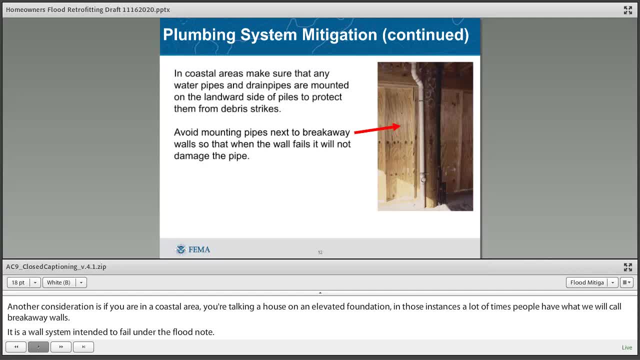 caused by the pushing or the lateral forces of those wave loads or high velocity water loads. And so if those walls break free, you are only getting down to those horizontal or lateral loads on the piles or columns. So that's a good thing when those breakaway walls fail. 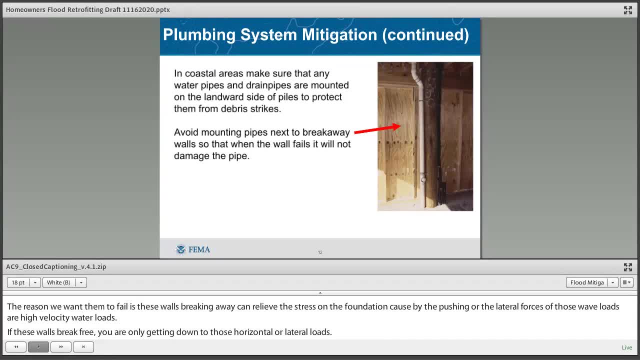 However, if you have a drain line like the one that we have pictured that could get hit by that rain, by that breakaway wall failing, there's two things that can happen. Potentially, that drain line could prevent the breakaway wall from properly failing. 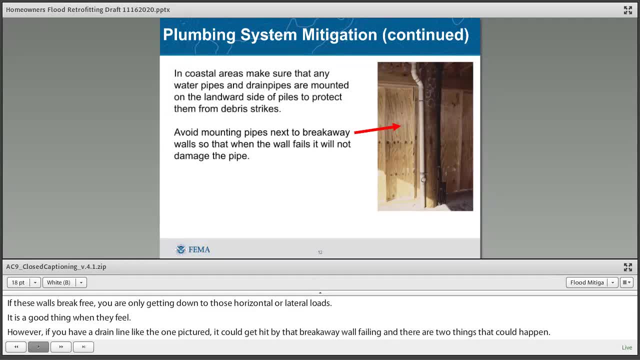 or the breakaway wall could damage or dislodge that drain line as it gets pushed away. So that's an instance where we want to make sure that we're going to mount that drain line in such a way that it isn't going to be impacted by that breakaway wall getting pushed away. 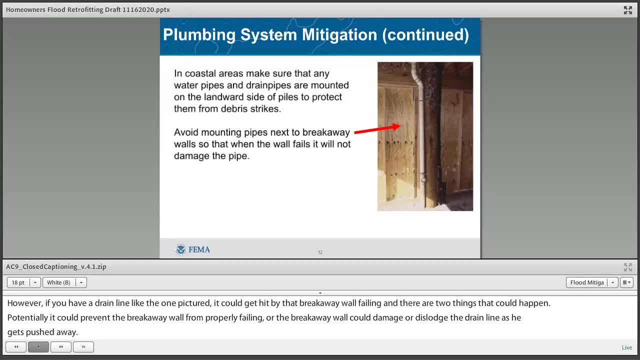 The other consideration that you have with these- and we'll discuss this really in the electrical section- is going to be the potential that you've got these drain lines or maybe electrical conduit lines that could be hit by debris if they're on the seaward side or the shore side. 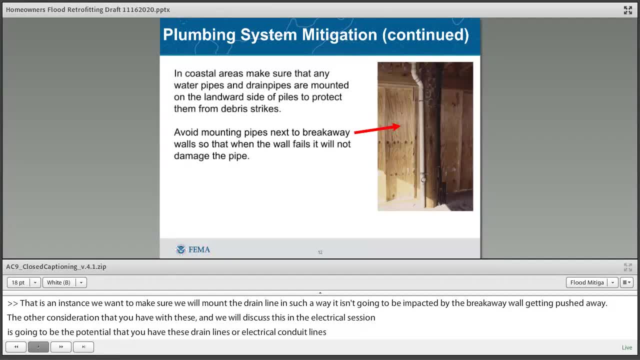 if you're on a coastal structure or if they're on the upstream side, the side that the water is coming towards the house from. if you're talking about a riverine location, We want to make sure that those lines are actually relocated around to the backside. 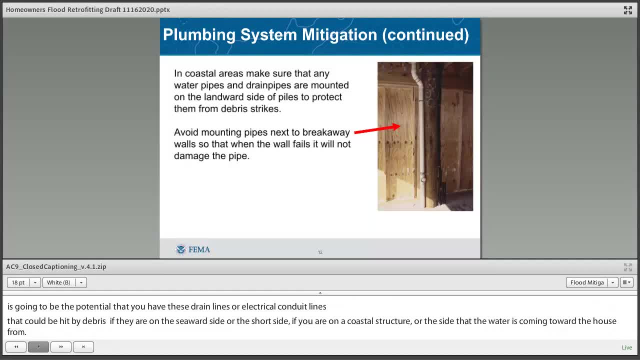 of those piles or piers so that they're protected And that way if debris is flowing downstream- so from upstream to downstream, or it's flowing from the shore to the land- that you can protect it. so you would want to mount those drain lines on the landward side if you're in a coastal area. 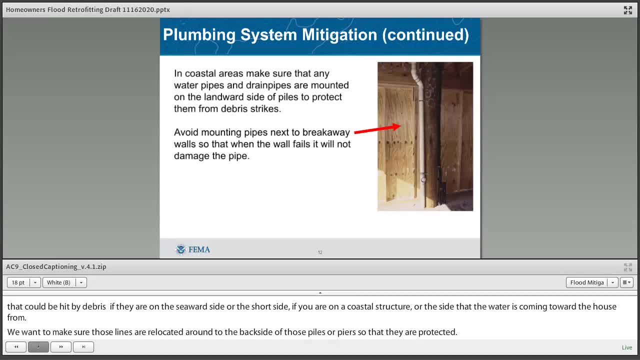 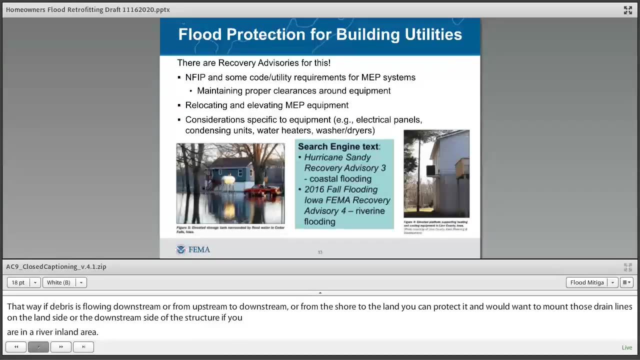 or on the downstream side of the structure, if you're in a riverine area, to make sure to protect those, because then that column, pier or a wall system can divert the water around that and keep that drain line from becoming dislodged. 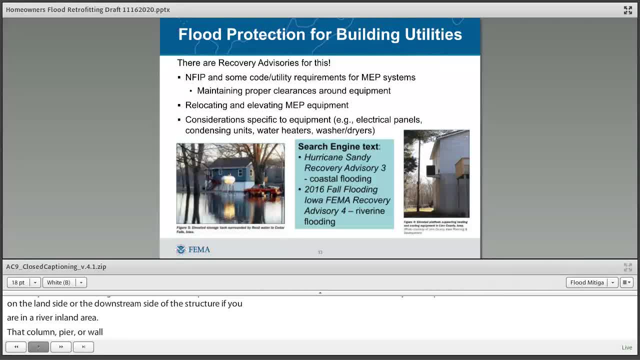 We have some recovery advisories on protecting we would call these building utility systems or mechanical electrical plumbing systems. That discusses a lot of the programmatic requirements with respect to the National Flood Insurance Program, as well as some code and requirements related to these types of systems. 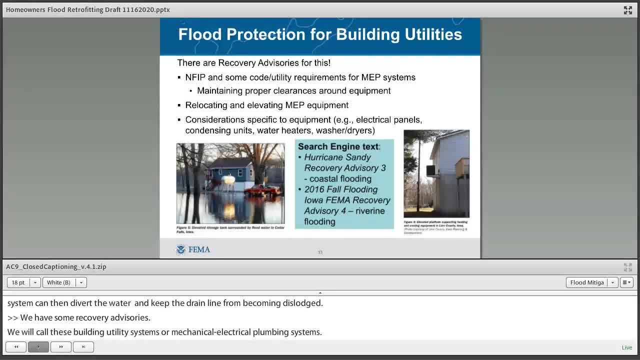 It discusses maintaining proper clearances around the equipment, the relocation elevation that I discussed and considerations for various types of equipment. If you're in a coastal area or subject to coastal flooding, we recommend using Hurricane Sandy Recovery Advisory 3.. If you're in more of a riverine location, 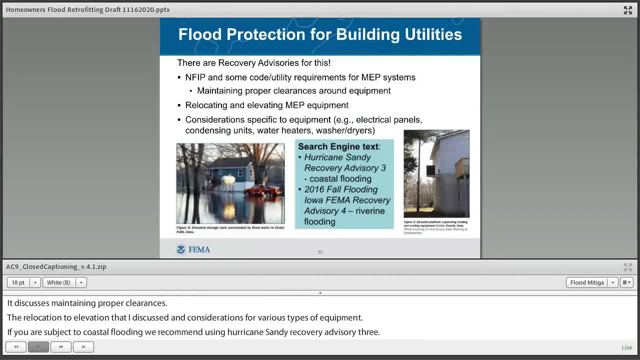 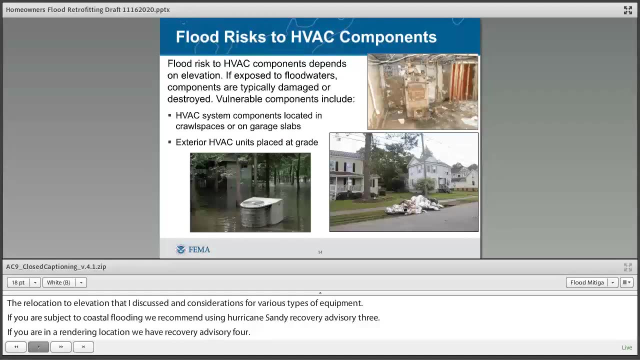 we have this 2016 Fall Flooding in Iowa, Recovery Advisory 4, and both of those you'll find are very similar, but they're sort of tailored to either a coastal flooding situation or a riverine flooding situation. Moving on to HVAC or heating, ventilation and air conditioning components: 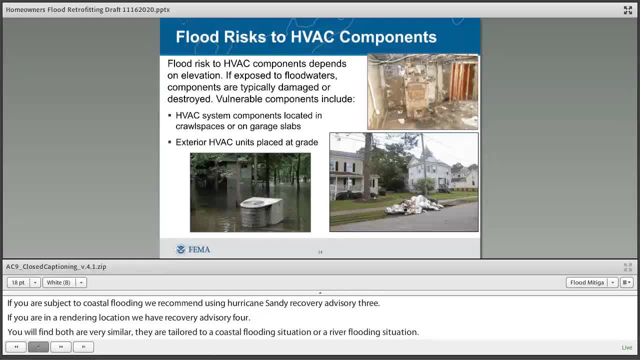 Moving on to HVAC or heating, ventilation and air conditioning components. Moving on to HVAC or heating, ventilation and air conditioning components: A lot of the damage that we see related to these is just the flood water touching these components and damaging these. 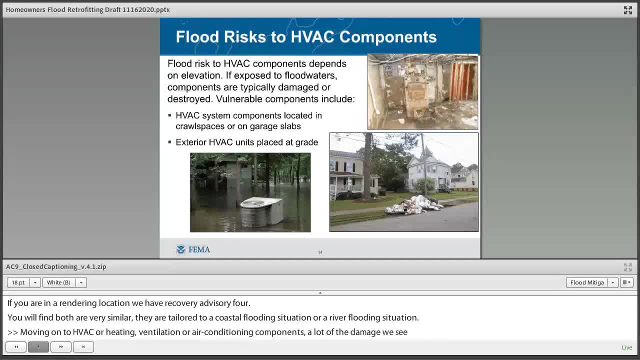 A lot of times. we have air conditioning units that are located right at the ground or just above the ground, on pads. We have heating systems that may be located on garage slabs or in crawl spaces, as well as the ductwork. So you'll see in the top right photo. 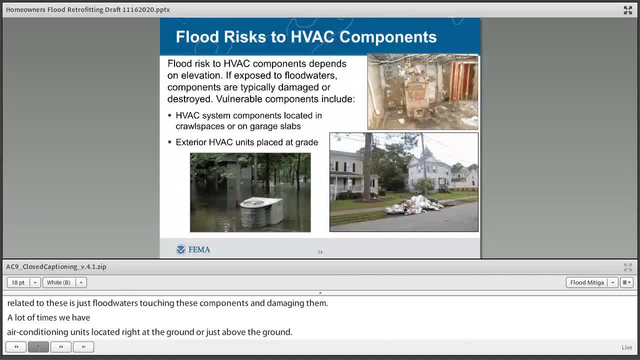 we've got a heating system that was in the bottom of a house. This is actually from Hurricane Sandy, but you can still see the flood water got in and it completely inundated the heating system and so that took that offline for the building. 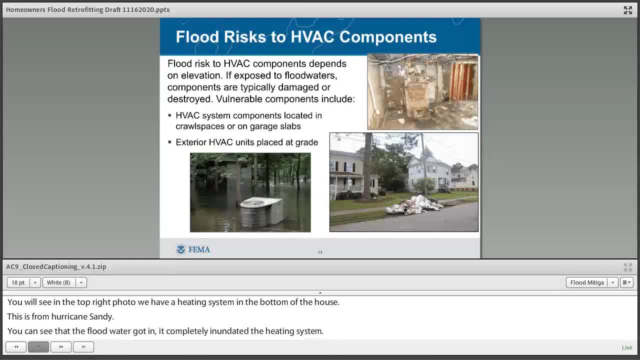 In the picture below that on the lower right. you'll see this is actually from Hurricane Florence in North Carolina. You'll see, this is a building that had a lot of ductwork underneath the house and the floodwaters got up. The floodwater didn't necessarily get inside the house. 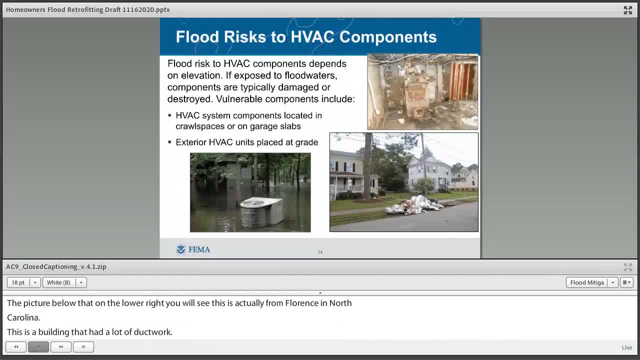 but it completely saturated the ductwork that was underneath the house, so they're going to have to remove all of that Now, if we think back a little bit about drawing out the house. one of the things when you run an air conditioning system. 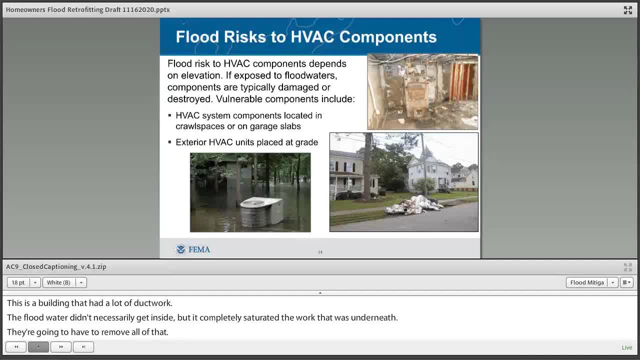 that it's going to do is remove the humidity out of the house, which that's going to help dry out the house quicker, But if your system is taken offline because your ductwork or your unit is flooded or taken offline, then you can't do that. 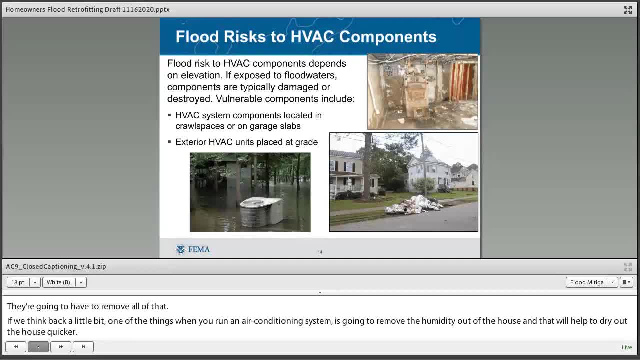 So that's one of the other reasons why it's really important that you get these units as high as possible, And this other picture on the left is an air conditioning unit that was located too low, probably on a ground-level pad, When those floodwaters came up. 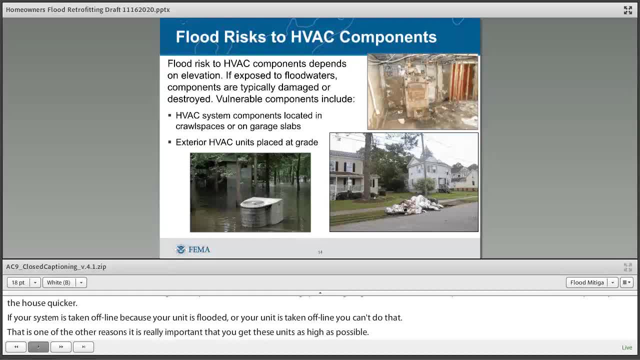 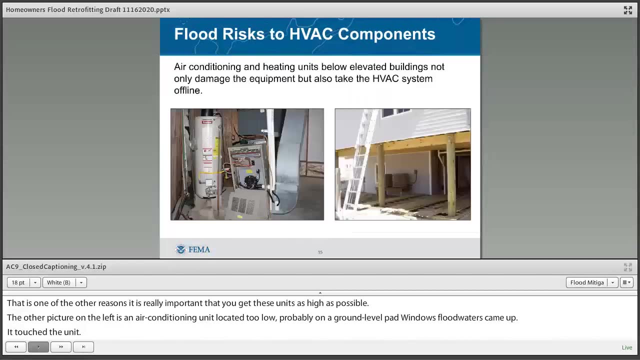 it touched the unit And remember how many contaminants are in it. Think about all the electrical systems, all the copper coils and everything that are in these systems, and just the corrosion that can happen when floodwaters touch these units, And so you're going to have to completely replace a unit. 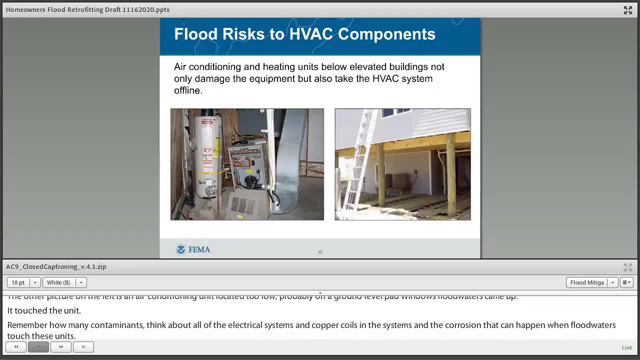 that gets inundated by floodwaters. Again, these air conditioning units are often below buildings. The picture on the lower left is just like we've kind of discussed before. It's actually a water heater and a heating system next to each other, And this was a coastal building. 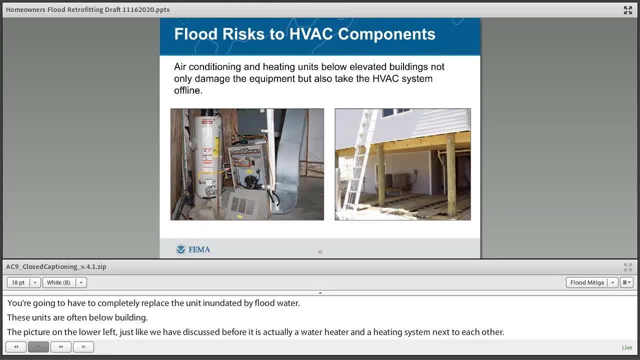 And both of those were inundated, taking both of those offline. And then we have another coastal structure on the lower right. This is a house that was elevated on piles but they did not elevate the air conditioning compressor, And so That can take that offline. 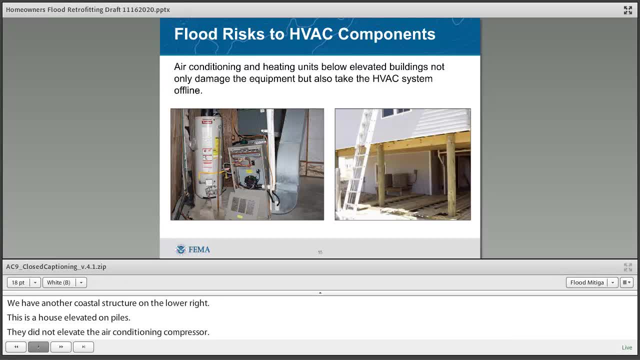 as well as if you're on a heat pump system, that outside compressor unit is going to act as both your air conditioning and your heating, And so that's going to take both of those units offline by having been inundated. So the reason why we want to move these units- 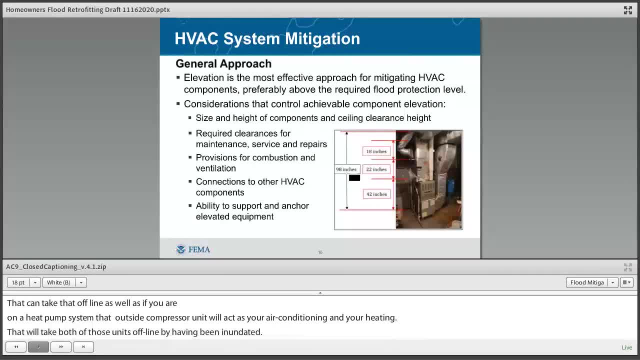 as high as possible and not take them offline. So the general approach, again similar to the plumbing, is to elevate these as high as possible, preferably above your minimum required protection. This is your base flood elevation, plus whatever additional requirements your community has. 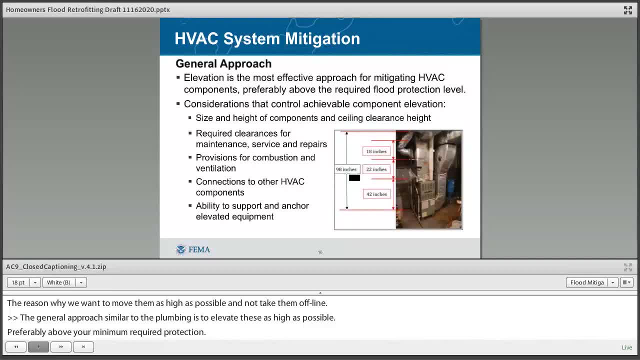 That's a really good idea. Often communities are adopting these higher-level requirements because they see that there's maybe an increased flood risk, So that's why it's a good guideline. But we want to consider sort of all the things that happen when we start to talk about it. 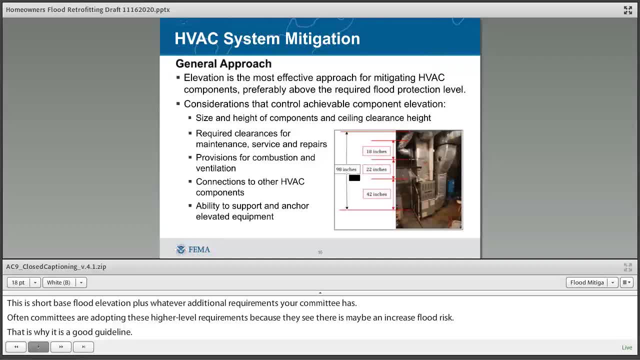 We want to look at elevating or relocating equipment. There's the size and the height of components, clearances that are required, provisions that are within the codes and standards for combustion and ventilation, making sure that basically, everything is going to be exhausted. 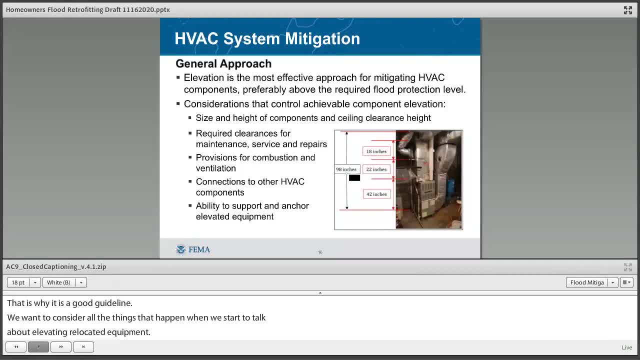 out of the system properly connections to other HVAC components- so maybe heating systems or maybe air handlers or ductwork, that sort of thing- and making sure that all those work together and then properly anchoring it once you've elevated it, to make sure that if anything moves. 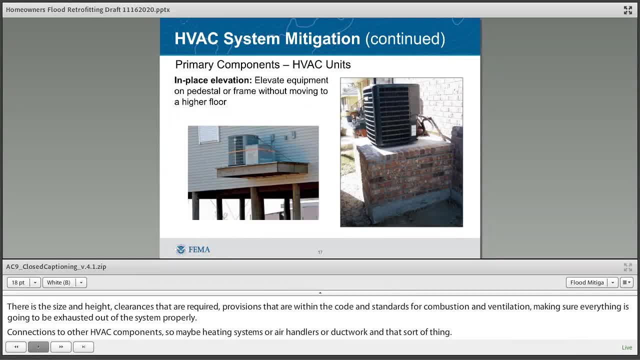 that that equipment is not going to be dislodged and fall. So, looking at elevating in place, here's two ways we've seen people elevate HVAC units. So here's what we refer to as a cantilevered platform off a coastal structure. 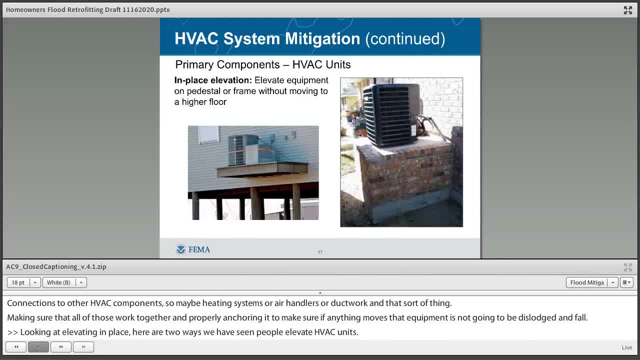 This means that they have no supports underneath it and there's nothing from a debris side that can damage that. and we'll show you an example of, if you have supports underneath that, what can happen if they're not properly designed. so this is an ideal way. 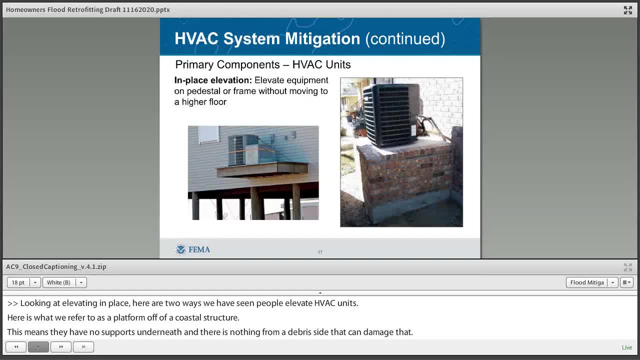 The other thing that they've done is they've properly anchored those units to that platform. so you'll see that they've got straps around those units in order to make sure that the wind isn't going to blow those units off. The other example that we have is on the right. 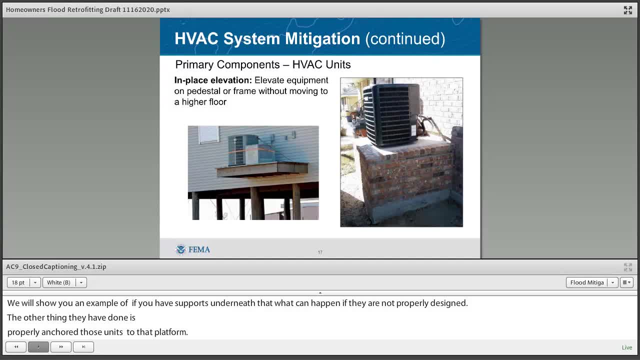 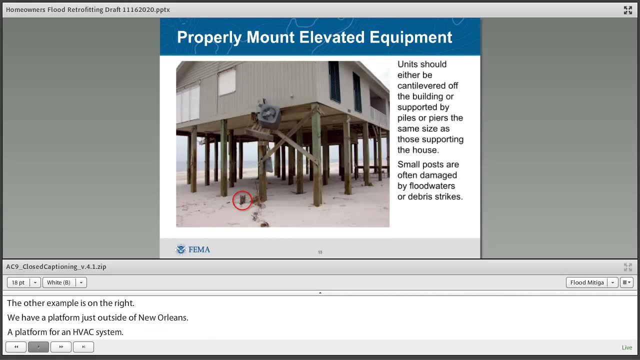 We've got a platform- This is just outside of New Orleans- just a platform for an HVAC system, and this gets it up above that minimum flood elevation that they were looking to protect against. So if we do have a platform on the outside of an elevated house, 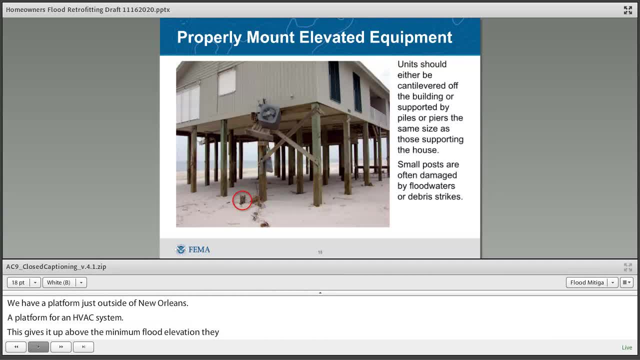 those supports should be the same size as the supports on the house. The problem is is that often we see people using smaller supports, so maybe they're using only a four-by-four post to support that platform. I mean it doesn't weigh much. 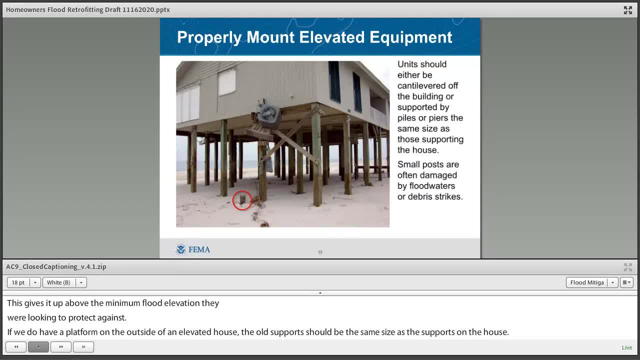 so people think I probably don't need a very big support. but we often see debris flowing in. That may be debris from your neighbor's house or something like that, or some debris from offshore or somewhere else in your neighborhood, and that debris gets pushed around. 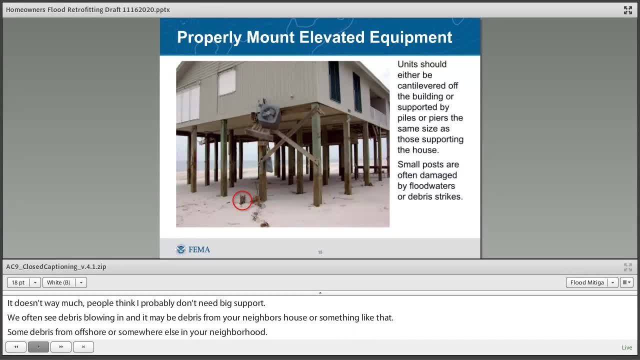 it takes out those posts and then, once that platform fails, then you've pulled the unit off the side of the house and then you've damaged that unit. So this is why we say you need a really robust support system or cantilevered system. 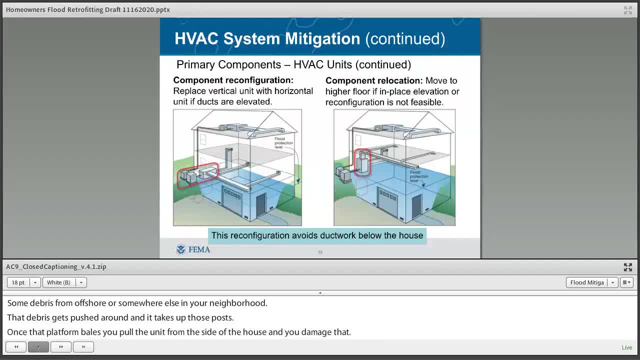 So if we're looking at relocating this equipment- this is an example in the lower right of a unit, that's where the ductwork is below the first floor. So we're looking at reconfiguring that, maybe from this style unit. 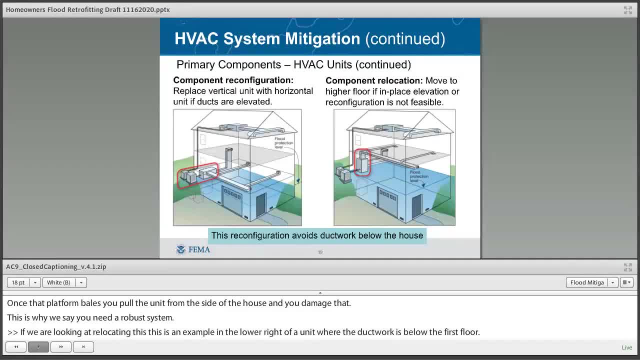 to the unit on the right, where they've gone to from more of a horizontal-type unit that's below the first floor system to one that may be in a utility closet or an old coat closet or something like that, and they've gone with more of a vertical unit. 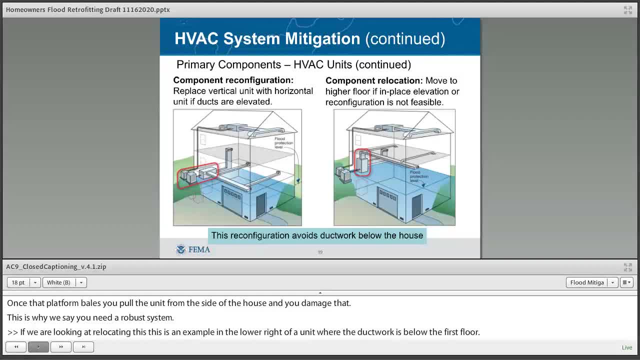 The thing that they were trying to accomplish with this is to remove the ductwork and that heating unit from underneath the house and bringing that unit into the first floor. This means that basically the main- we would call it the trunk- line, where most of the airflow moves through the house. 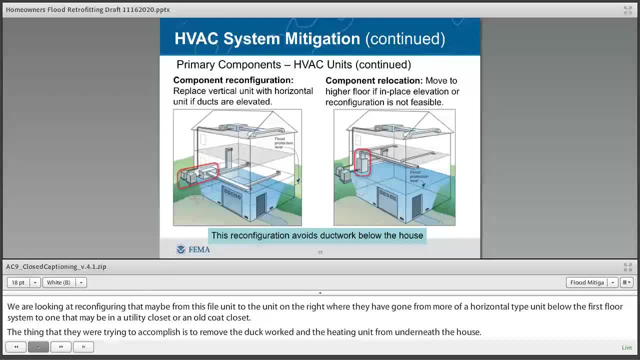 they actually had to build sort of a- we would call it a soffit below the ceiling system, but they had to run it just right at the ceiling system and sort of box that area out to just finish off that ductwork, so you see just drywall or something. 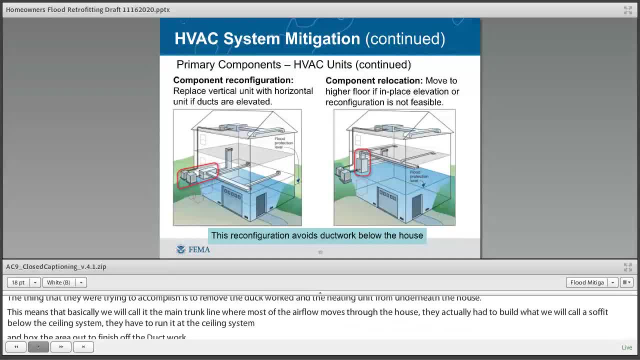 rather than anything else, It's just exposed ductwork. But then the lines that are actually running out to the registers that you would feel the air blowing out of those are run through the ceiling system or the floor system. for the second floor That's run through there. 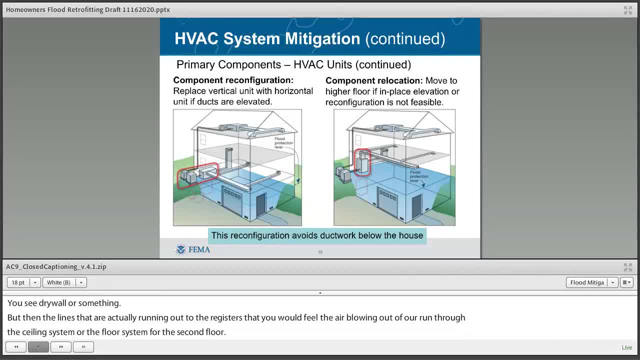 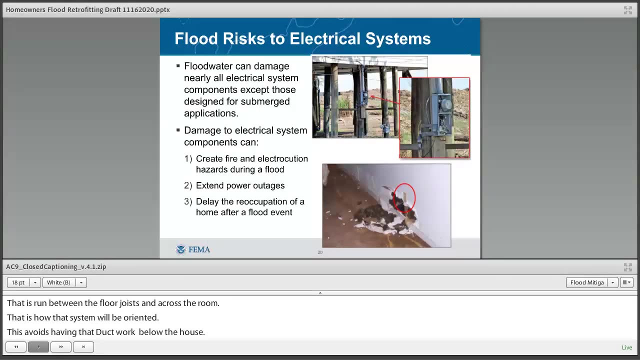 between the floor joists and run across the room. so that's how that system would be oriented. But this avoids having that ductwork below the house and if the floodwaters touch that, you're having to rip all of that out. so that's the intent of this effort. 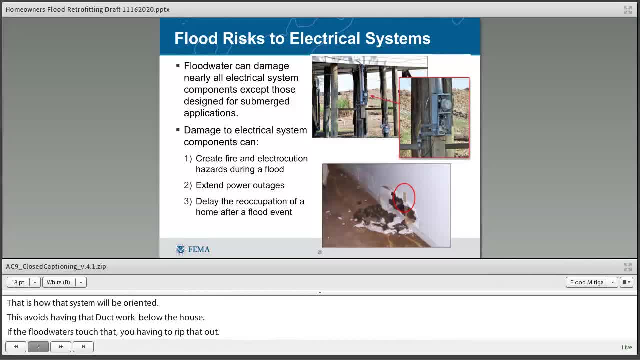 Moving to electrical systems. flood damage can will basically damage anything that it touches. Flood water, as well as a storm surge from the ocean, has either the salt water or lots of other contaminants in it, and so, once it touches electrical equipment, the smartest thing to do is to just replace all of that. 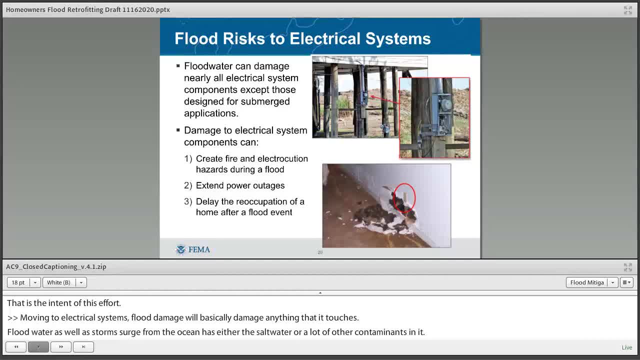 It creates a fire and electrocution hazard, as well as causing, you know, outages in the house, and it can delay reoccupation of the house. so we want to try and get all of this equipment as high as possible, The thing that we want to try and think about. 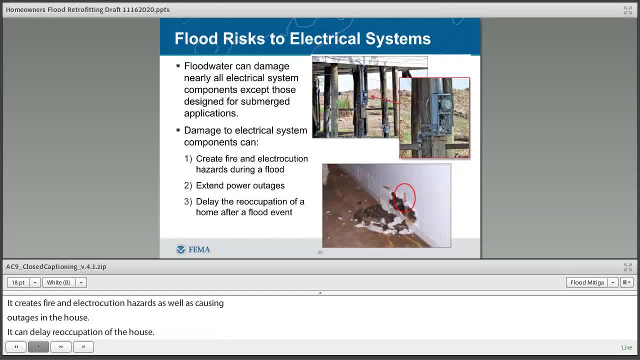 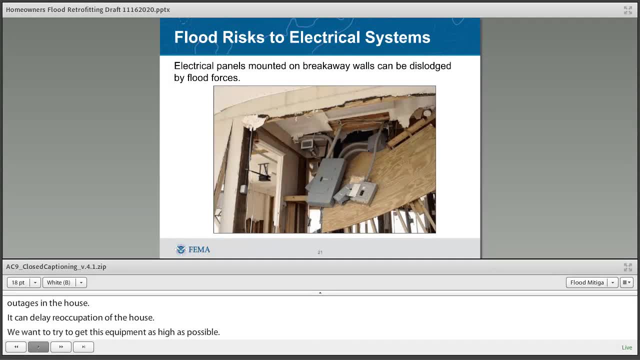 is just making sure that everything is as high as possible and that you're not going to end up with taking the whole system offline. So the other thing that we discussed, or that we will discuss as a problem, is going to be that if these electrical panels 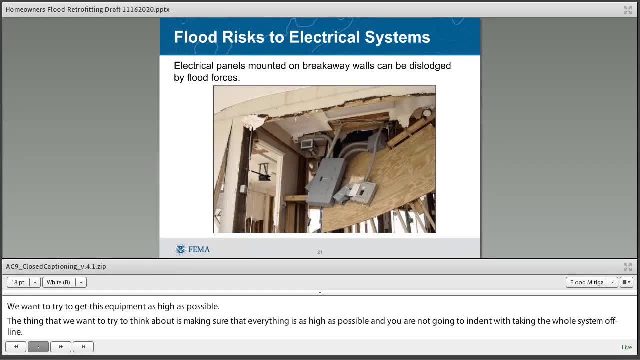 or any of the electrical meter maybe is attached to a breakaway wall, that if that wall breaks away during that flood that it can do a lot of damage. Not only is it taking that electrical system offline, but that electrical system may prevent it. 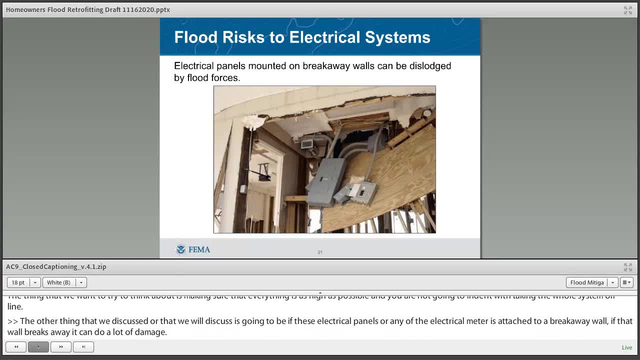 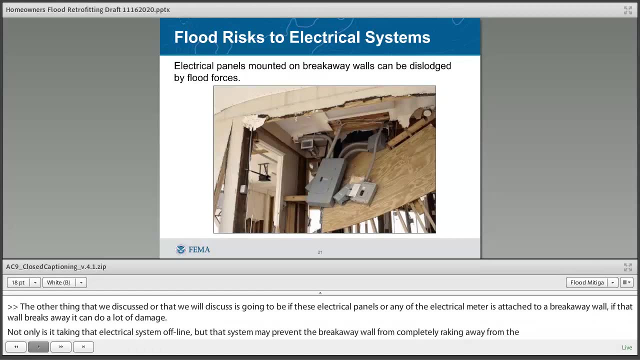 from taking the whole system offline. That electrical system may prevent that breakaway wall from completely breaking away from the pile or column that it's attached to, and so we want to make sure that, basically, once that breakaway wall breaks away, that it's completely breaking away. 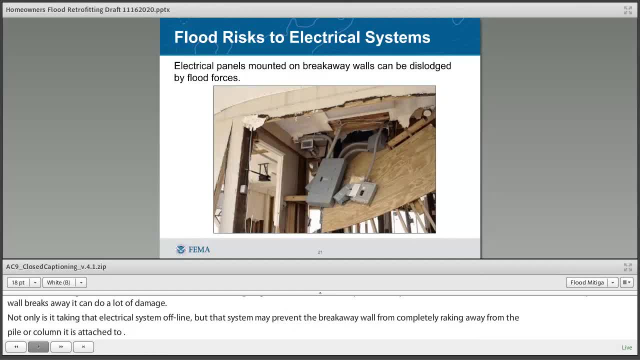 and that it doesn't pull all this electrical system with it. So if you do have breakaway walls, you want to make sure that all of these units- the meter, the electrical panel and everything- is up in the house and not attached to this breakaway wall system. 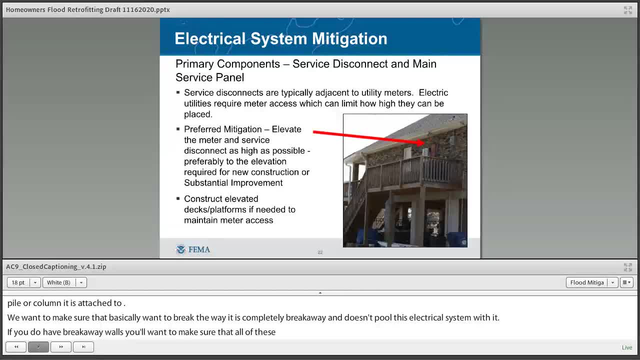 The main components that we often see damage to are the meter and the main service panel. So ideally, what we want to do is try and get those as high as possible, ideally elevating the meter and any sort of service disconnect as high as possible. 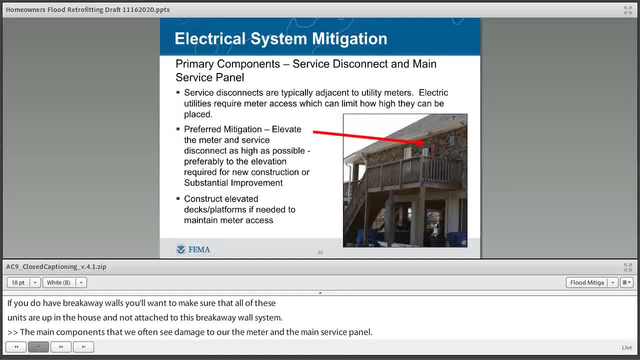 You'll see this picture. We've got an arrow to where the meter is located. You'll have to check with your electrical utility about whether they will allow you to elevate these- Some utilities like them- on the ground approximately four or five feet above the ground. 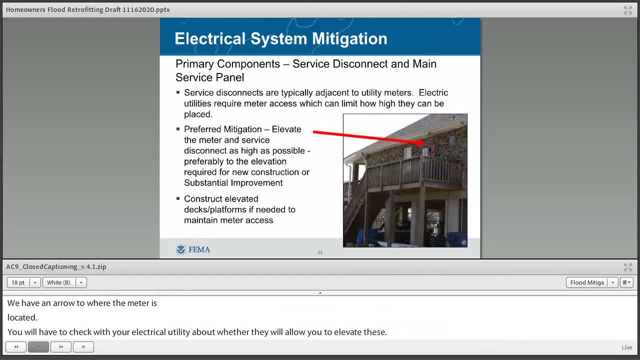 Others will let you relocate them up to a deck area. What they try to discourage you from doing is building a platform just for that electrical meter. Often they like to have it on the same deck as the electrical meter as the main entrance and exit to the house. 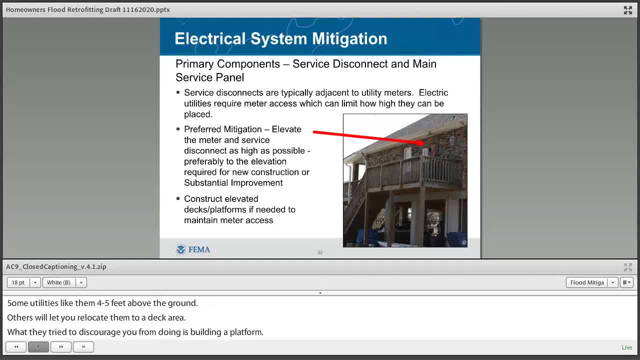 So you'll see, this one is located by the front door and this means that with the panel up there, that the intent is that the utility expects that the homeowner is going to maintain that deck system, versus a separate deck system or separate platform system that may not get maintained as well enough. 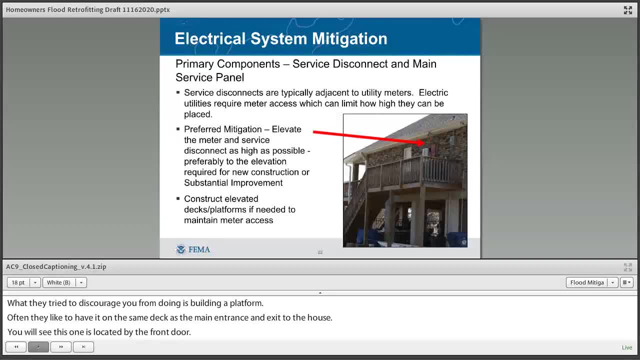 and then you may be putting that utility worker that has to go and access that at risk. So that's why they really try to make sure to either have them located from ground access or somewhere that they know can be maintained, because we don't want those utility workers. 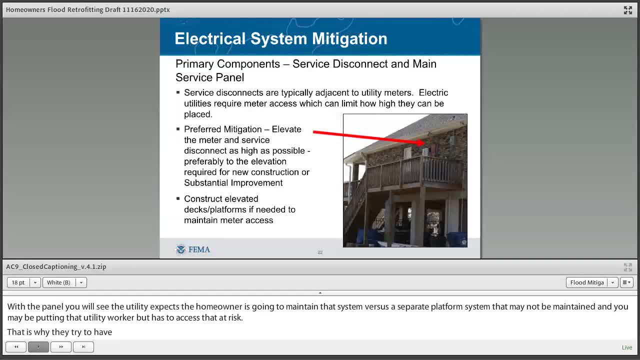 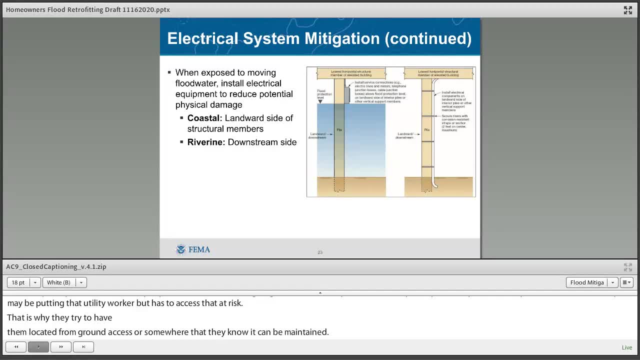 to be put at any more risk than they already deal with in their day-to-day job. So, just like we discussed before with the drain line, this is an example of a picture showing you that both the electrical meter and any lines, whether that's an electrical conduit line, 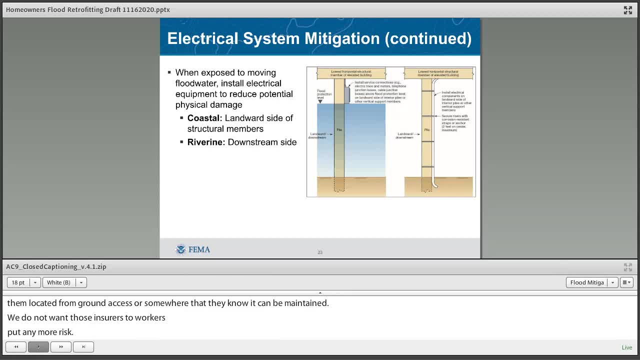 or a drain line for the house, those should be located on the downstream side. if you're in a riverine situation so the water is pushed around that pile and not going to impact that electrical meter, or if you're in a coastal area, that it's on the landward side. 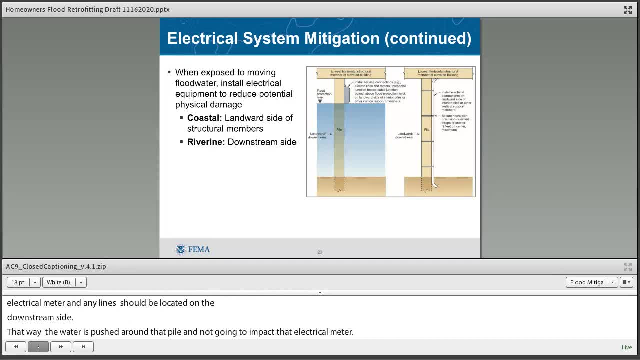 so that when the storm surge comes up that it's again being diverted around the pile or post. This is a good example. in this diagram on sort of the left view, you can see that they elevated the panel as high as possible or the meter as high as possible. 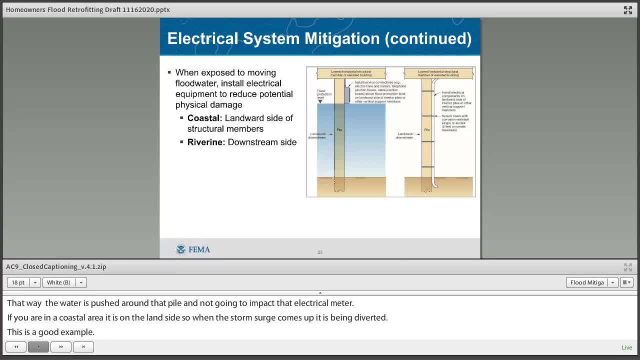 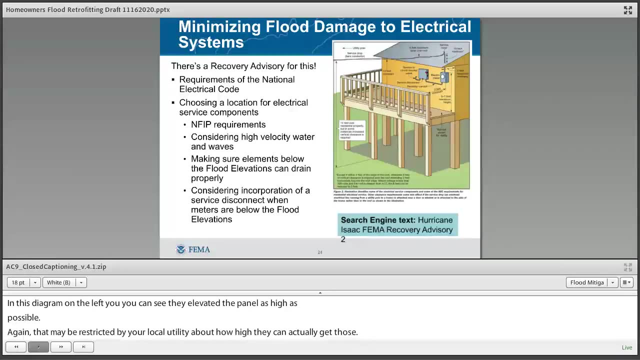 but again that may be restricted by your local utility about how high they can actually get those, because they want them to be available for a utility worker to look at without having to get up on a ladder or anything. so you may be limited on how high you can get those. 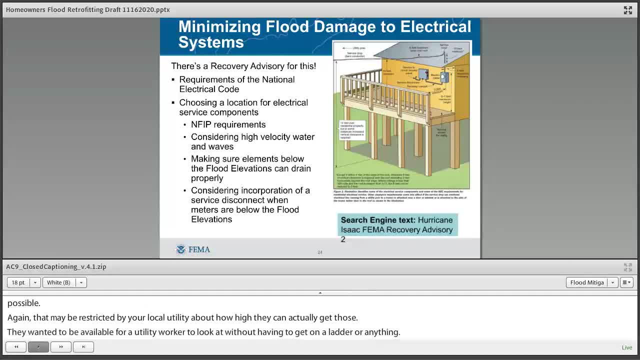 We do have a recovery advisory that talks about all of this stuff that I've just touched on. This is Hurricane Isaac Recovery Advisory. 2. This discusses portions of the National Electric Code, the National Flood Insurance Program requirement considering high velocity water and waves. 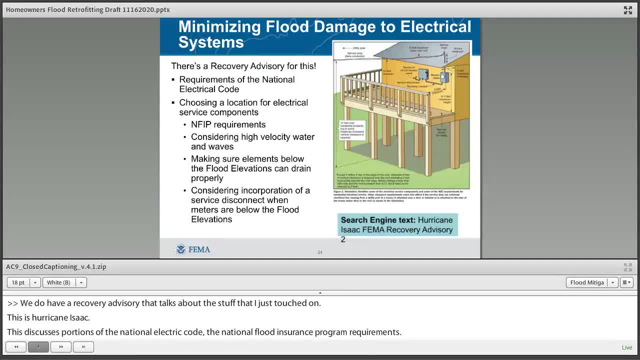 and looking at elevations. One of the things that we kind of encourage people to do when they're looking at this stuff is maybe if you've got any elements of the electrical system, from a safety standpoint, that's below this elevated building, so maybe just some lights or something like that. 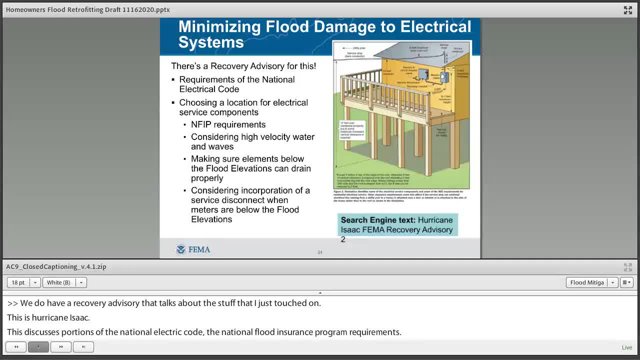 that's required for safety in an enclosure below this elevated building, that maybe those are on a separate circuit breaker from the rest of the house, so that if those were damaged and needed to be isolated that you could just turn off that circuit breaker and still maintain power to the rest of the house. 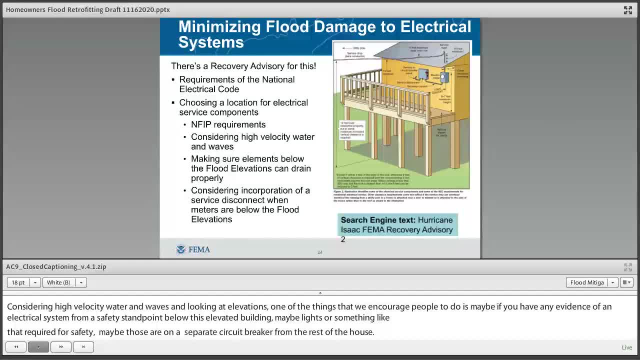 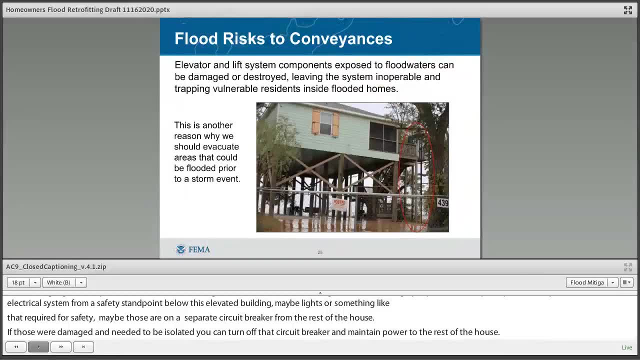 So the other thing I would consider as much as possible is trying to isolate any electrical lines that are in these areas that you're at risk for getting touched by flood water. Just briefly, looking at flood risk 2, we call them conveyances. These are elevators and lift systems. 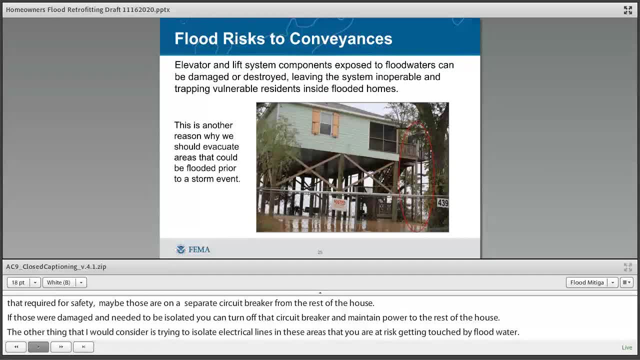 A lot of times, the equipment can get damaged, or the actual lift that you're riding in can get damaged, And so those can get taken offline. This is another reason why we tell people that they should be considering evacuating If you have mobility issues. 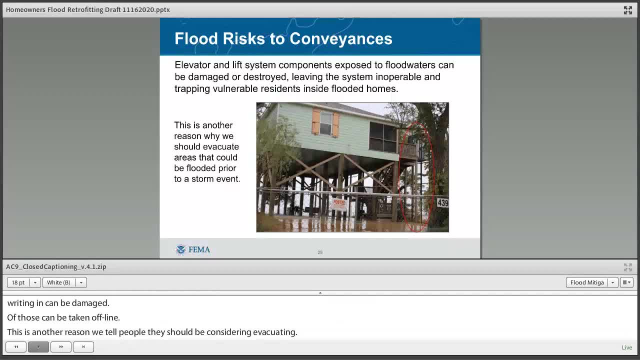 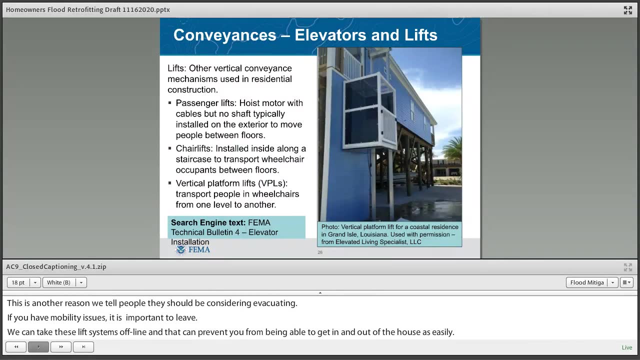 then it's important to leave, because we can take these lift systems offline and that can prevent you from being able to get in and out of the house as easily, and you may be having to use the stairs for long periods of time. So we do have some recommendations on this. 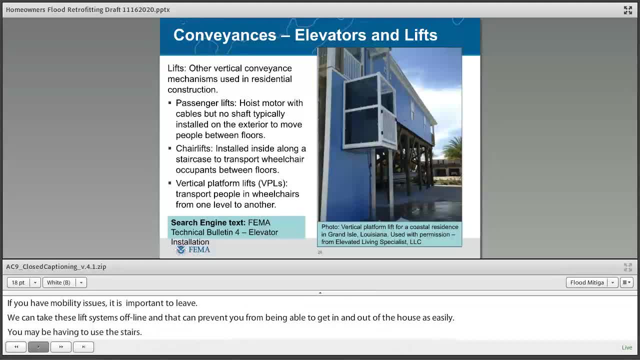 FEMA Technical Bulletin 4,, which is elevator installation, is a really good thing. In this instance. I would type in FEMA Technical Bulletin 4 versus elevator installation, because FEMA Technical Bulletin 4 is the exact document that you want. The other one's a little. 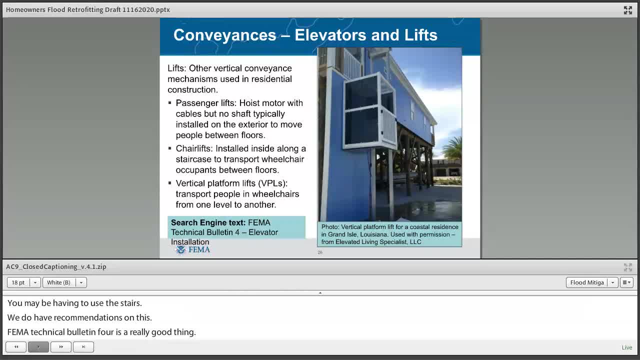 the title may be a little vague- from our search engine to find you the FEMA document we want you to use. This talks about just different guidance for passenger lifts, chair lifts and other vertical platforms to get people with mobility issues in and out of the house. 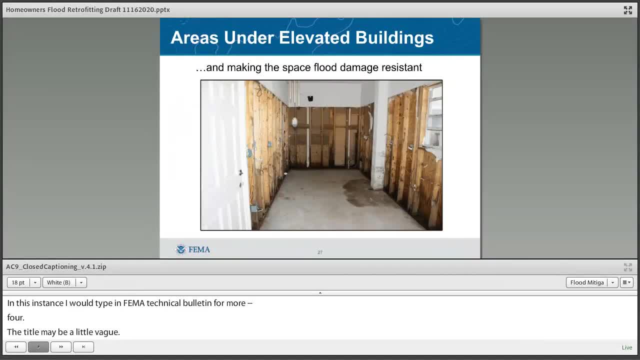 So some helpful guidance if you've got any of those on your home Areas under elevated buildings and making those flood resistant. This is a picture from Hurricane Isaac Plaquemines Parish. This was really a house, an area under an elevated house. 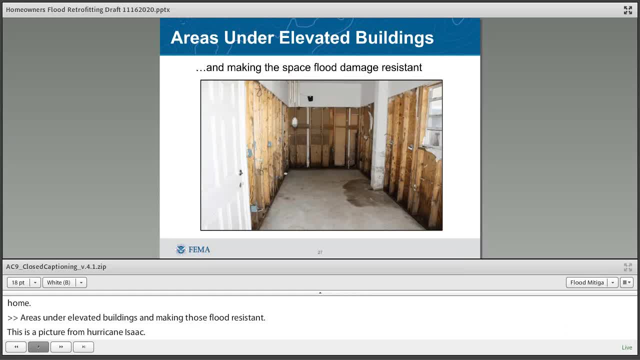 that was finished a little bit too much. You can see the gray electrical boxes that were all damaged by the flood waters. There was some plumbing damage and that sort of thing. So this was sort of an area under a house that doesn't meet compliance. 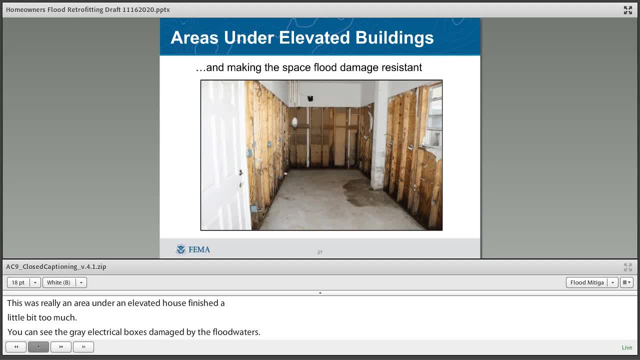 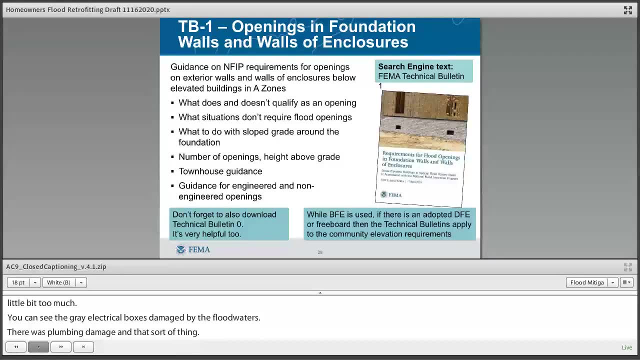 And you can see all the damage done as well as the drywall removed from all of these. So we want to minimize those and look at how can we prevent this from happening. So one of the guidance documents that we have is FEMA Technical Bulletin 1.. 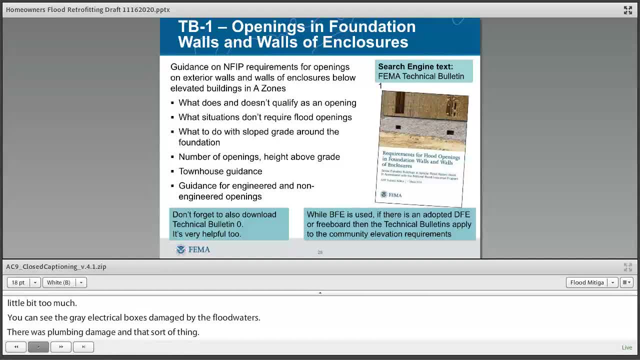 This is guidance on openings in foundation walls. You'll see the picture of the guidance document and you'll see those black openings that are the flood openings. Sometimes people refer to them as flood vents, but this is guidance on that. What does and doesn't qualify as an opening? 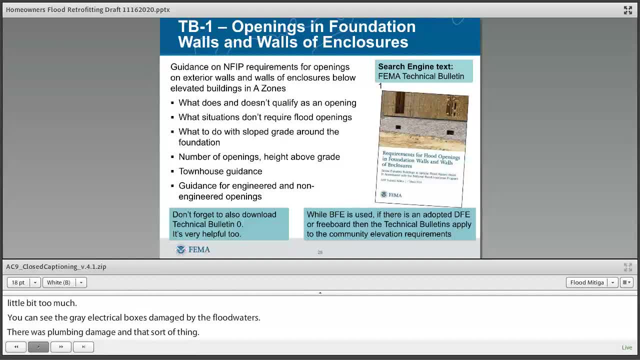 What situations don't require flood openings. What to do if you have a sloped area around your house? The number of openings and the height above the ground. What to do if you have a townhouse or something like that And there's two types of openings? 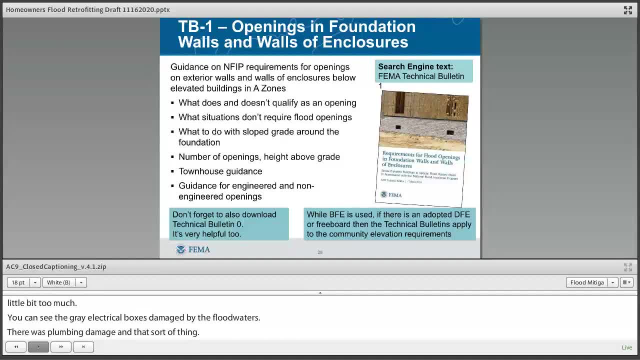 and it goes into basically engineered, which are the ones that maybe have the flap that moves up and down, versus non-engineered, which is just the standard sort of opening. There's nothing behind it. The base flood elevation is used for these, but if you have an adopted design flood elevation, 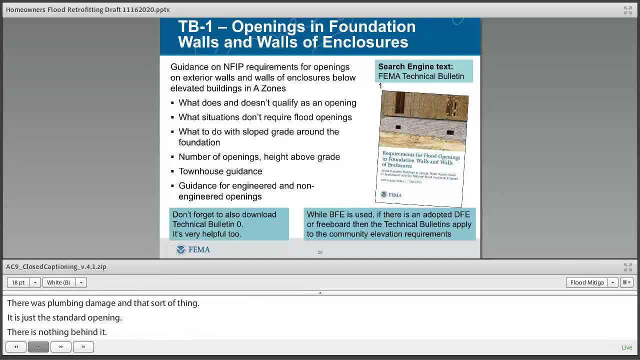 or there's freeboard, as we talked about, one foot, two foot above that base flood elevation required by your community. then the Technical Bulletin does not require or discusses how to apply those. I would also say: don't forget to download Technical Bulletin Zero. 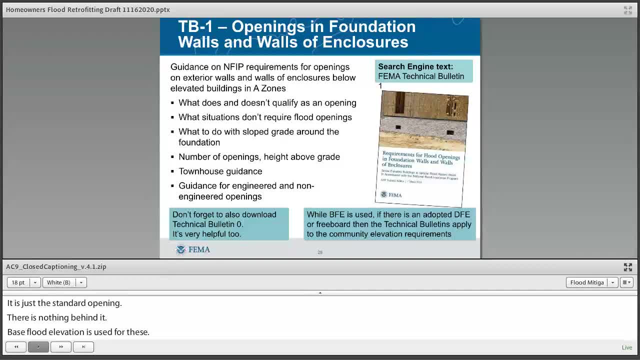 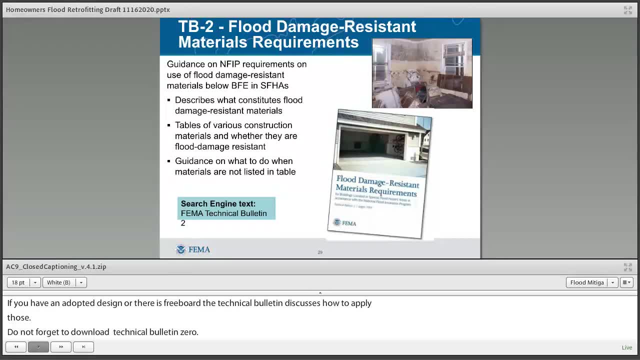 Technical Bulletin Zero has a really helpful acronym list as well as defining a lot of the terms used in the Technical Bulletins. Technical Bulletin Two is on flood damage resistant material. This is guidance on materials that you can use below the base flood elevation if you're in a special flood hazard area. 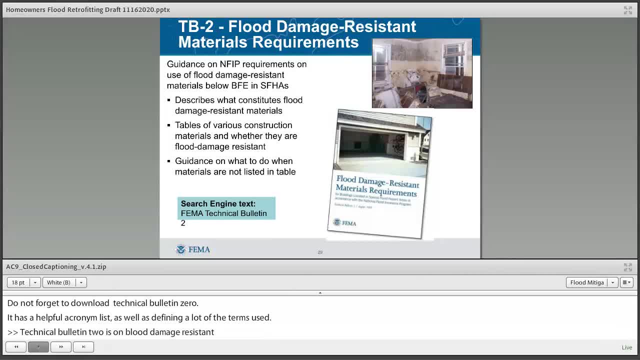 It describes what constitutes flood damage resistant material. It's got a table that lists the type of material, lists where that material is used. Is it used for a wall system or a floor system or a ceiling system kind of thing? It also lists how resistant. 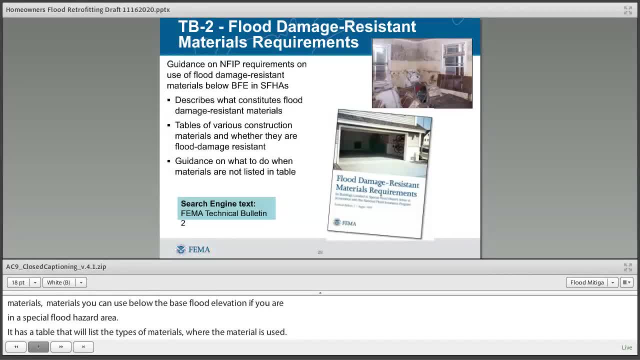 to flood damage? is that material? This guidance also provides you a list of what to do when materials are not listed in the table, So how to take if you're dealing with your local building official on a material that's not listed in the Technical Bulletin. Two: 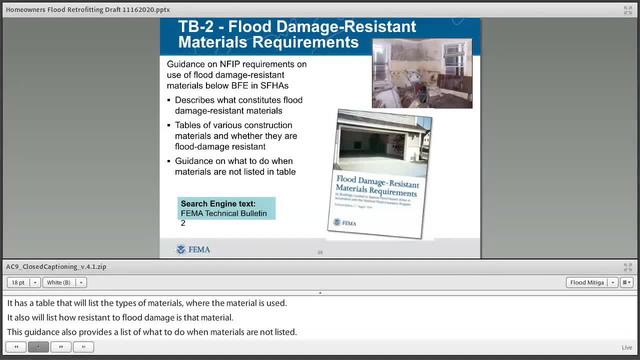 what type of materials that you need in terms of technical specifications from the manufacturer in order to have that local official make a decision. Ultimately, the decision if it's not listed in that table is up to the local official. So in all the instances with whether a material 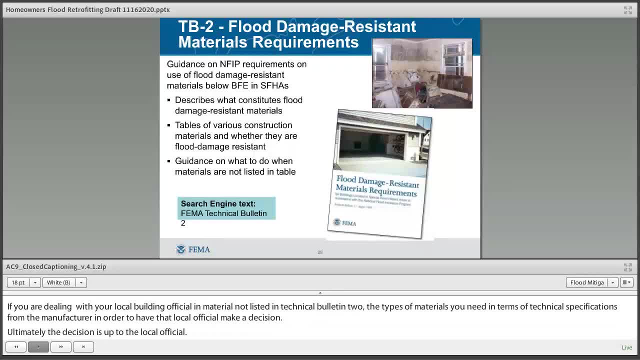 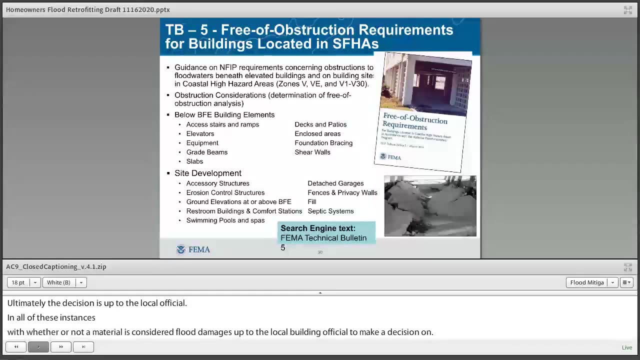 is considered flood damage resistant is up to the local building official to make a decision on, since they're actually the eyes on the ground for this program and making sure this program works. So it's at the community level that those decisions are made. If you're in a coastal area, 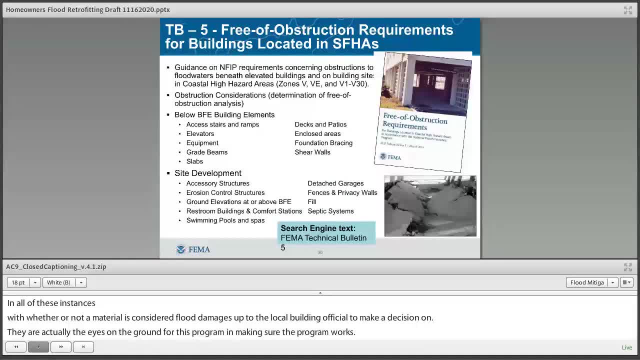 Technical Bulletin Five. this is free of obstruction requirements. Some of you may know that you're in a V-zone or a high velocity area. This is areas where we have large waves and fast moving water, and it provides Technical Bulletin Five, provides you what we would call free of obstruction. 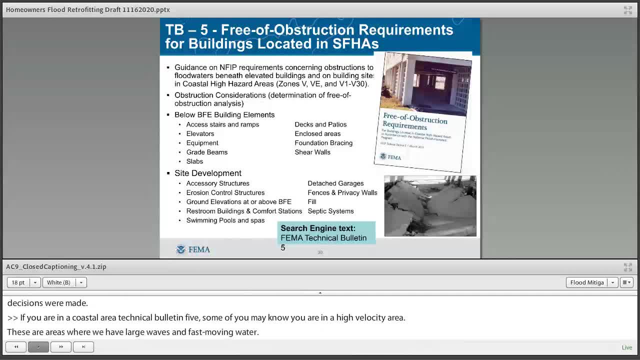 sort of what is an obstruction, how to consider it, how to do an analysis if you want to put something in, maybe a pool or something like that, how to address those considerations that are required in order to make sure that you're not going to do damage. 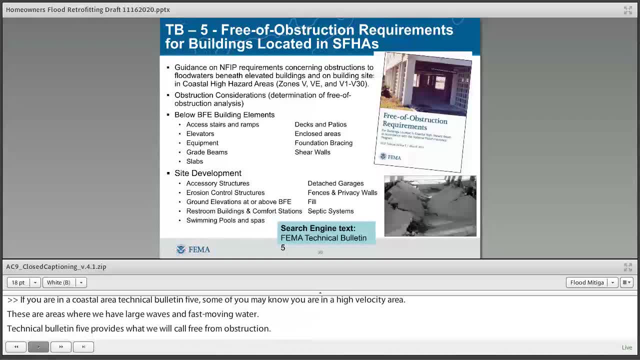 not only to your house, but also your neighbor's house. That's kind of what free of obstruction is about. This talks about several building elements, things like stairs, elevators, parking slabs, decks, patios, that sort of thing. 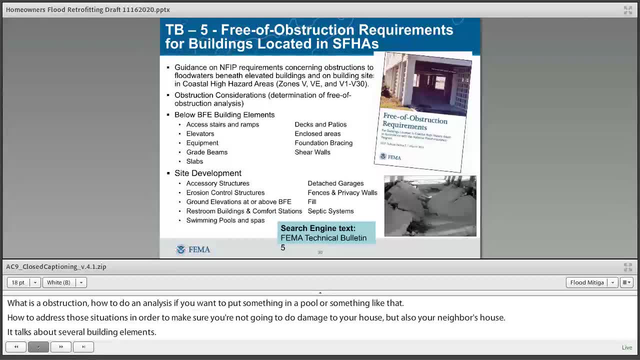 foundation bracing sort of how to do all of this properly, as well as site development. This could be accessory structures, detached garage fences and that sort of thing, pools and those sorts of things around buildings and just looking at making sure. 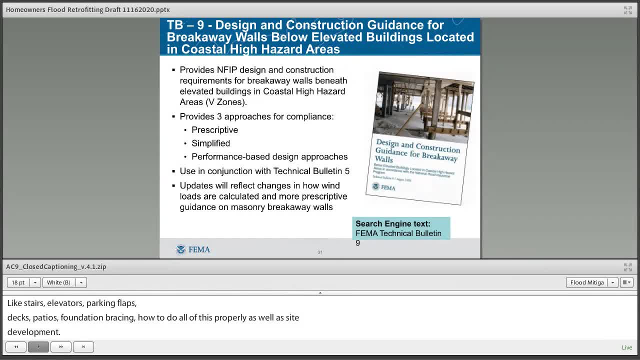 that those are going to be compliant. Technical Bulletin Nine. we've talked briefly about breakaway walls. This provides breakaway wall guidance and gives you three approaches: a prescriptive, a simplified. So these are going to give you sort of guidelines on how that would be framed. 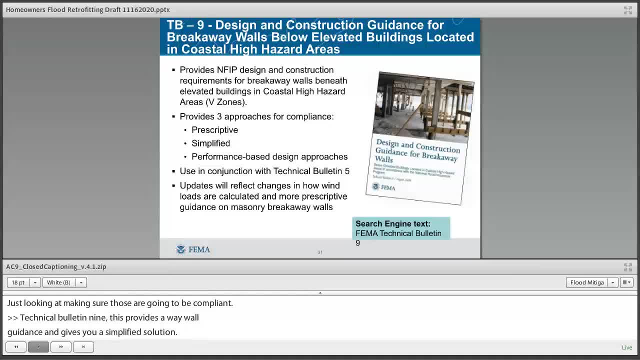 in terms of a wood frame wall And then performance-based design approaches. if you don't meet the criteria for the prescriptive and the simplified, what's another way to get an engineer or architect to design those systems for you and gives them guidance? 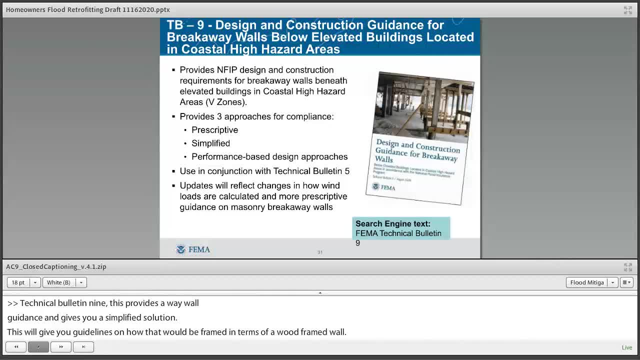 It's going to be used in conjunction with that Technical Bulletin Five that we just touched on, And we're currently in the process of updating it, but I think for a lot of a lot of architects and engineers they can work off the old version. 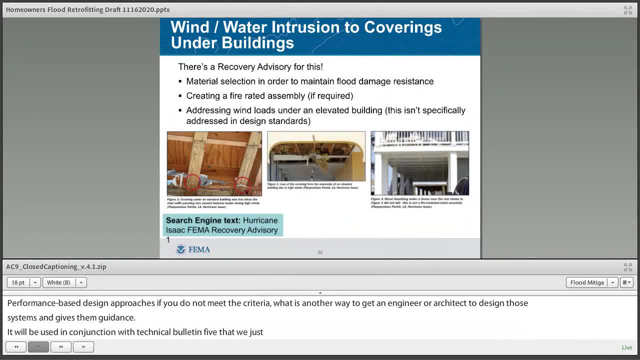 and come up with exactly what you need: Wind and water intrusion to coverings under buildings. So you'll see in the picture on the right, this is a, the covering underneath an elevated building. Now you may have a garage area or something like that too. 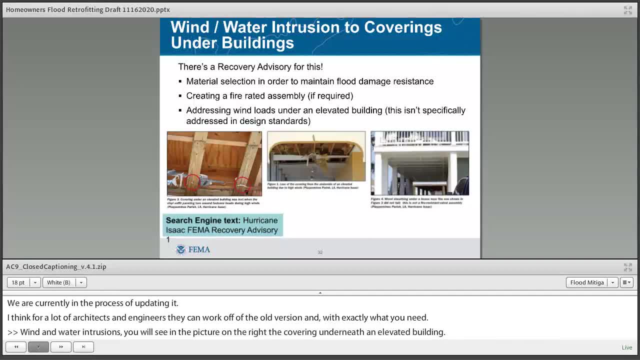 And so we've discussed, you know- how to deal with situations like that, because you're talking about an area that's exposed to potentially floodwaters, to high wind and then the other hazard that you may have if you're parking or doing anything under that area. 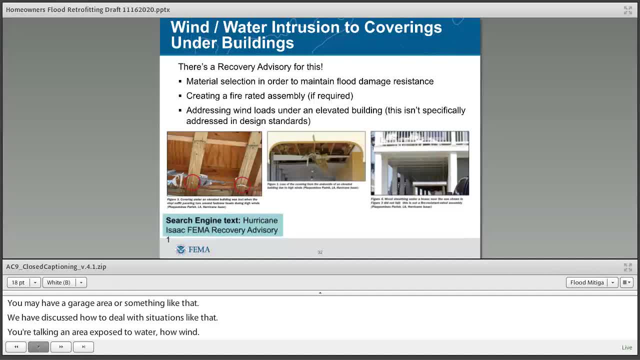 is the potential for fire, so fire resistance to that area. Often we're seeing people use vinyl systems to cover those areas. You can see in that middle picture that's a vinyl system that's been pretty torn up by high winds And then you'll see the picture on the right. 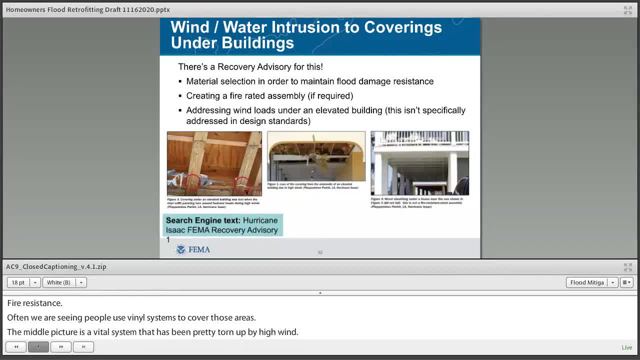 I'm sorry the left that has. there used to be a vinyl covering there, but the vinyl was pulled out from around the nail holes and so that vinyl system is completely gone. Now why do people have these systems? They're trying to protect the insulation. 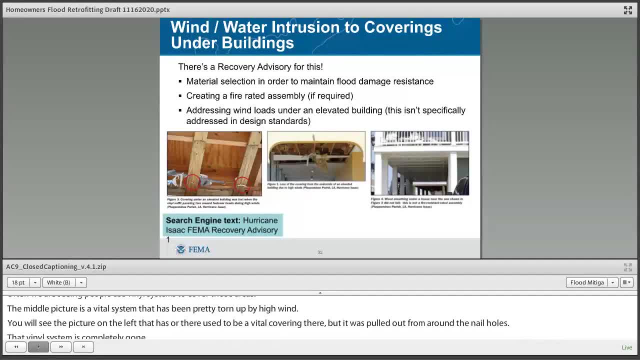 under the elevated buildings. so you know buildings up on piles or columns, But they're also protecting the wiring, the plumbing system, just whatever's underneath that house is trying to get protected. So that's why we want to make sure that you have a good system there. 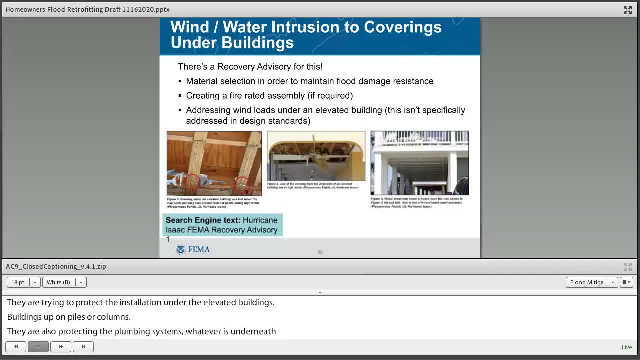 But if you need a fire-rated assembly, that's an assembly so that if, say, you're parking underneath this building, there's a fire with your car or something, that you have plenty of time to get out of the building and the fire department has time to come. 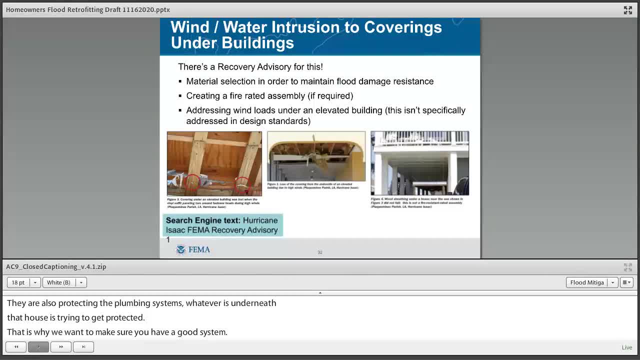 and that your whole building is not damaged by this, to minimize that damage. So there's what's called a fire-rated assembly. That's described in there, So that isn't just a matter of using some fire-resistant- uh, plywood or something. 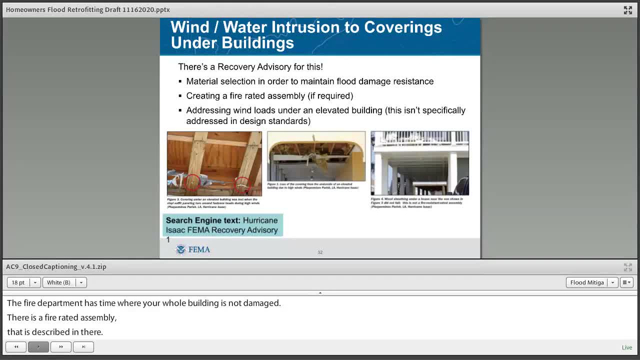 It's a matter of the whole assembly and trying to give you some time on that before, if there's a fire before the things on the other side of that fire-rated assembly are damaged. So that's covered, because we want to make sure that we had a fire-rated assembly. 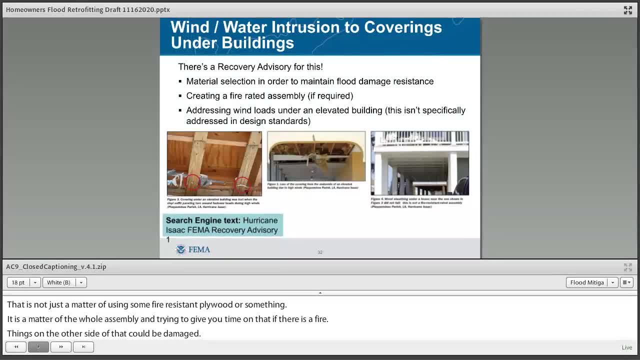 that was designed for high wind and flood. Um so, and some of these things are not specifically addressed. uh, specifically, things that we want to make sure that they're covered. Uh, specifically things like the wind in a lot of the design standards. 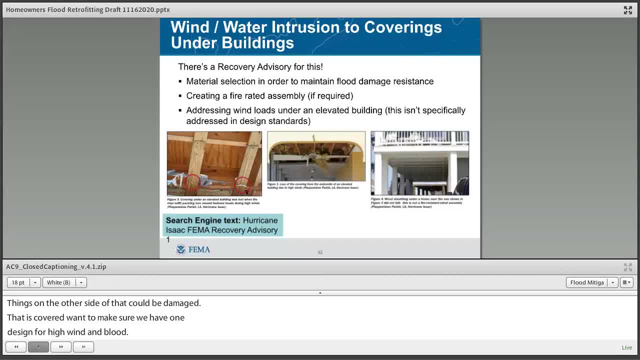 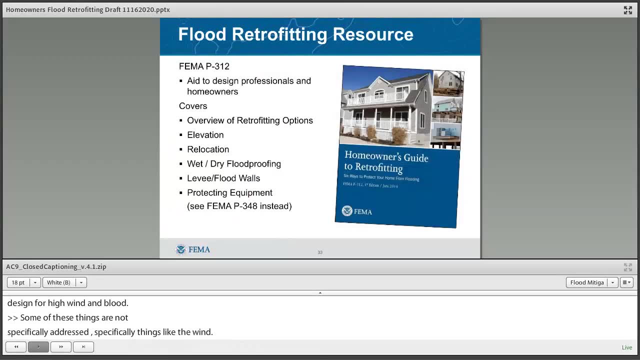 that we did the best we could with trying to describe how to address those situations where you'll get good performance out of um. these sort of soffit covers or covers over elevated buildings. Some flood retrofitting resources. FEMA 312 is the Homeowner's Guide to Retrofitting. 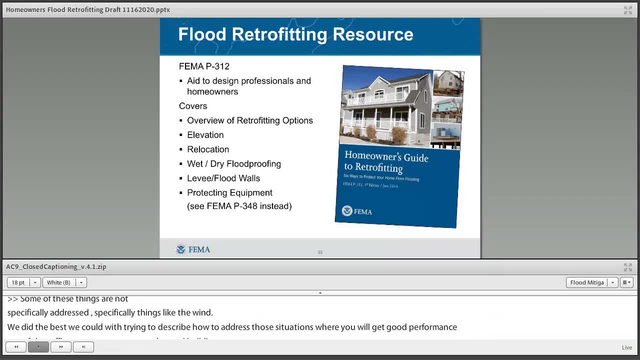 That kind of gives you six different options: Um elevation, relocation, wet-dry flood, proofing uh levees and flood walls. and protectors- Some flood walls and protecting uh equipment. Now, uh with these if if your house has been substantially damaged. 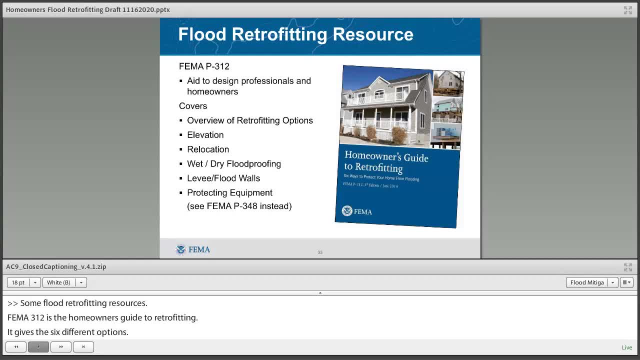 we would recommend that you look at elevating or relocating or or potentially just rebuilding the entire structure. Those are the recommended options. Wet and dry flood proofing: uh, they are covered, but we would really discourage you from doing those because, uh, dry flood proofing is basically. 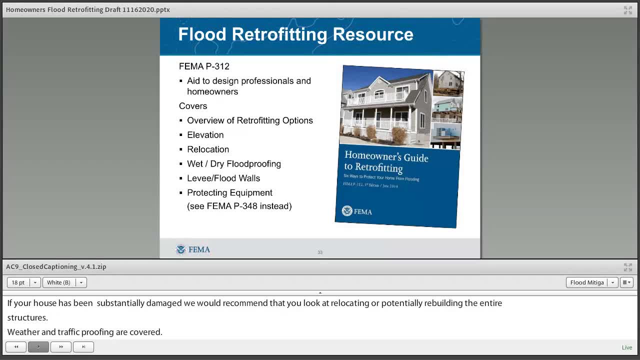 typically, people see that as wrapping their house or putting shields up over door systems and stuff like that. Potential for damage and catastrophic damage to the house is extremely, extremely high, and so we would discourage you from doing that. Uh the the water loads for dry flood proofing. 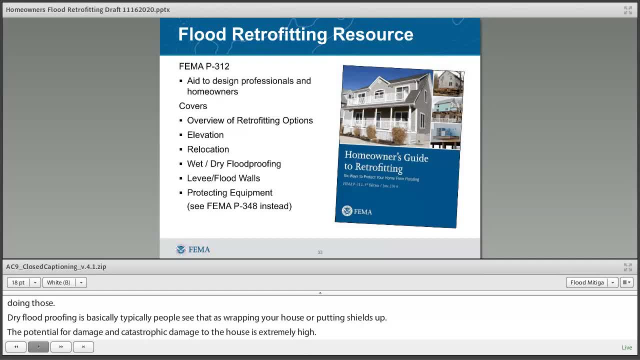 at home are extremely high. Uh, wet flood proofing is basically letting water in and out of the home. This is great if you're talking about uh areas below a house, but if you're talking about letting water in and out of living areas. 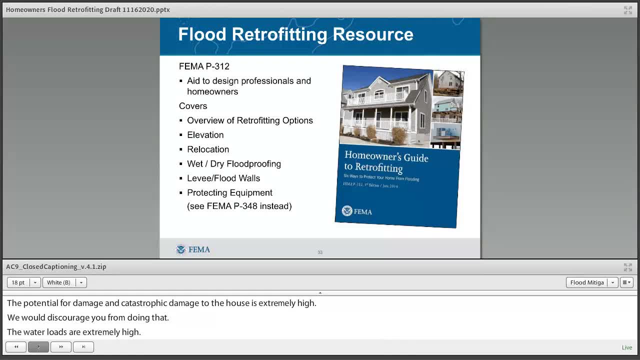 there's a lot of concerns with doing that, so we would discourage that also. Uh, the levees discussed in here are what we would call private levees, so not the the big river type levees, that that you uh see. 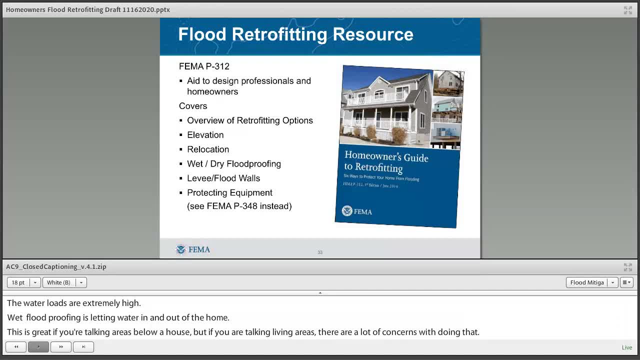 but these are maybe small berms around houses and that sort of thing. and what are the pros and cons of doing that? Um, flood walls. the same way, we're talking about small flood walls around buildings. These are mainly, uh, for minor flooding. 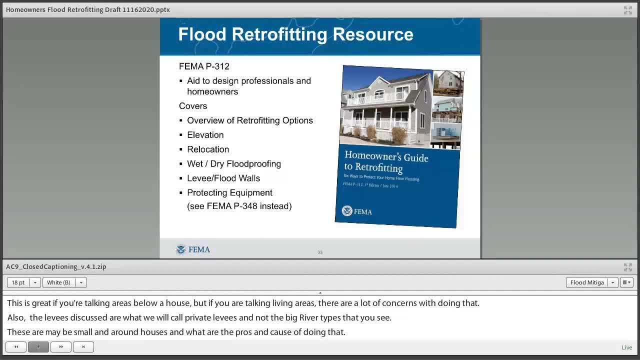 maybe a foot or two of flooding, but if you get very high with the flood waters, then really you need to just look at elevating the building because of the potential risk to your, your building. Uh, I would also say, before you consider, uh. 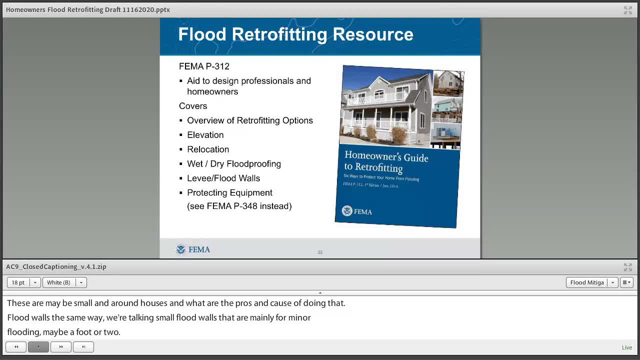 a levee or a flood wall. you want to kind of talk to your local floodplain administrator as well, as if you're looking at wet and dry flood-proofing, I would talk to a local official about that before you do that. Just somebody that could come out. 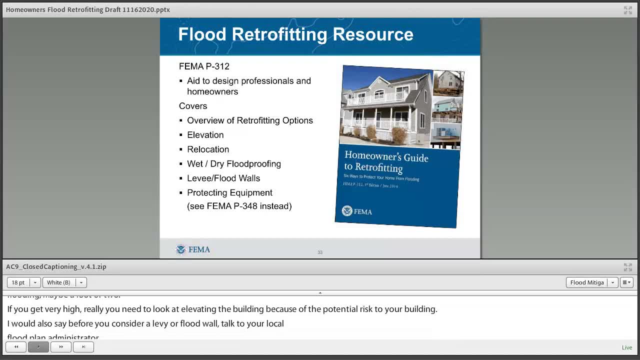 and and look at your building and and kind of explain what the risk really looks like. Protecting equipment- this is mechanical electrical plumbing system. We'd really recommend you use FEMA P-348.. Uh, that, that's a more recent one. 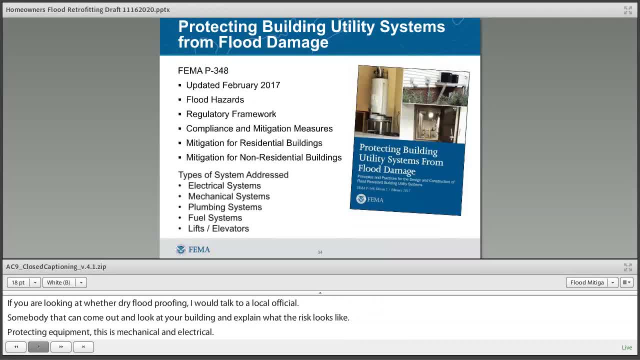 It's a recent publication and I'm about to discuss that. FEMA P-348 is really your go-to resource for looking at mechanical electrical plumbing systems. Uh, we cover sort of what flood hazards do. uh, what, what do the regulations look like? 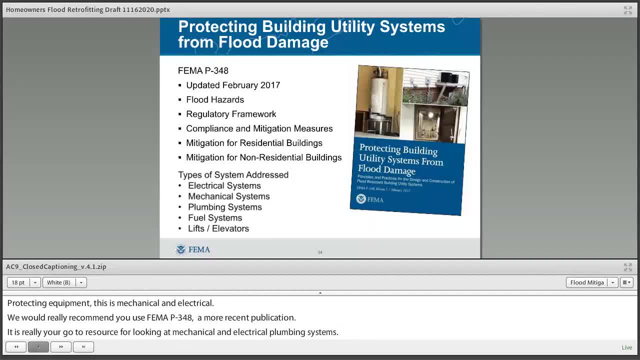 uh what is considered compliant? We talked about compliance and meeting uh those uh regulations and requirements earlier, so we talk about uh what compliance looks like. Uh, there's a section for uh mitigating residential buildings. 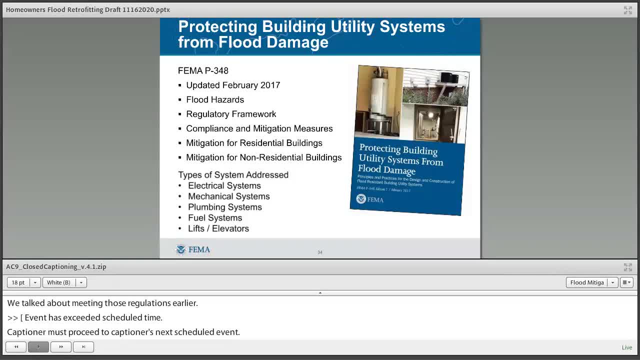 so your single-family homes as well as non-residential kind of commercial-type building, And we cover electrical systems, mechanical systems, plumbing systems- Something we didn't cover in this course- fuel systems. so that's uh, your propane tanks. 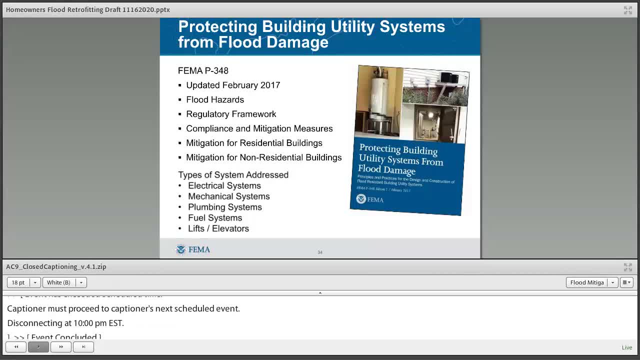 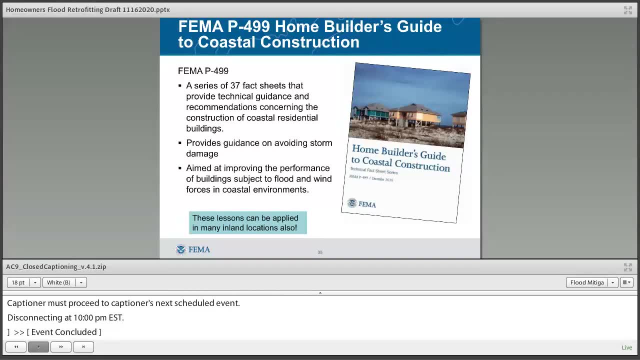 and that sort of thing. so that's really helpful to have that in there as well as, uh, the other item we discussed, conveyances, which are lifts and elevators. Uh, an another group of fact sheets. uh, this is FEMA 499.. 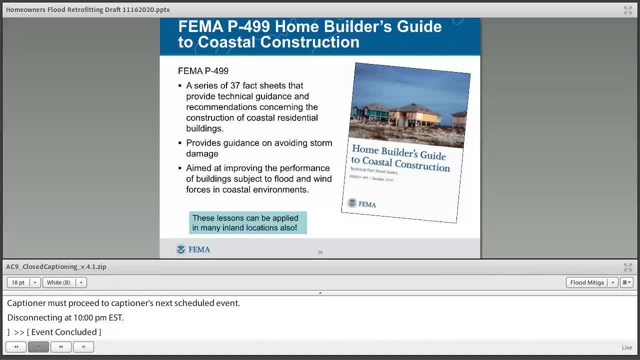 Um, these are the Home Builders Guide to Coastal Construction. Uh, this is 37 fact sheets. The thing I really like about the Home Builders Guide to Coastal Construction is the fact that it it gives you some really helpful guidance. uh, that are individual fact sheets. 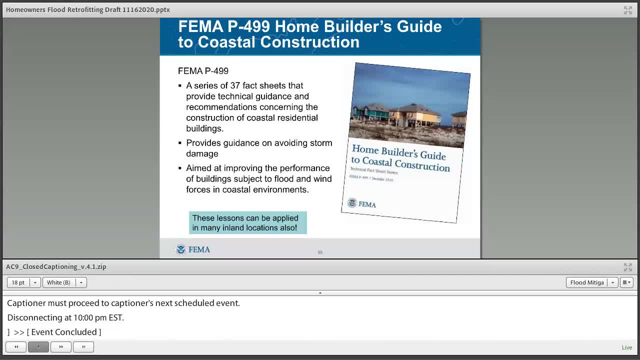 So maybe you've got a uh one specific problem. Maybe maybe you're looking at your wall systems, or maybe you're looking at windows, or maybe you're looking at flashing or something like that. Uh, there's fact sheets specifically on that. 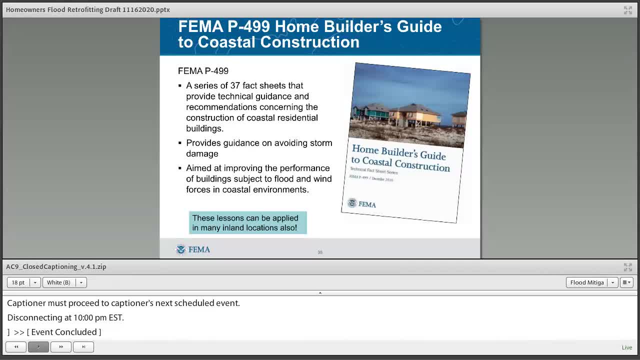 so you can hand those to your contractor and have your contractor kind of go through and see exactly what we're recommending that they do. Um, even though this is coastal, a lot of those lessons can be really helpful for inland communities. so I would say across the board, 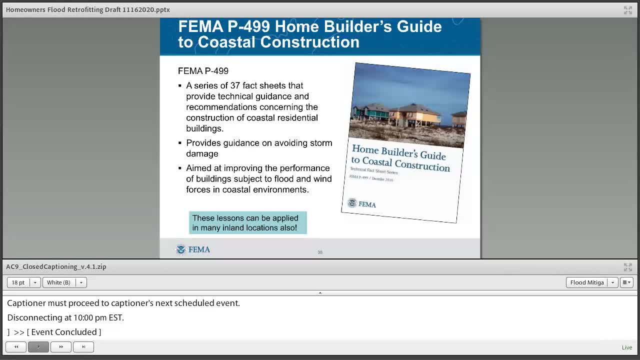 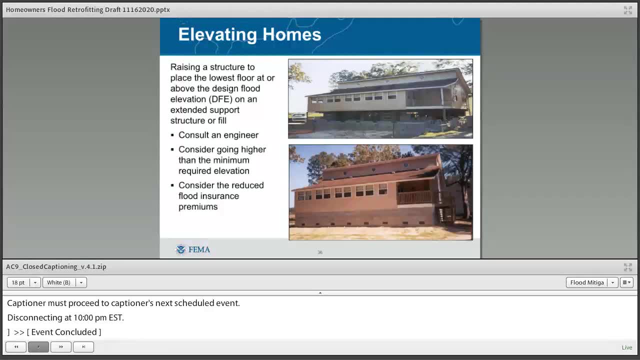 if you are subject to hurricane risk, that this is really gonna be a helpful guide for you, even if you're not like right along the shoreline, like the picture is showing on the cover of it- Uh, elevating homes. I'm gonna touch on this briefly. 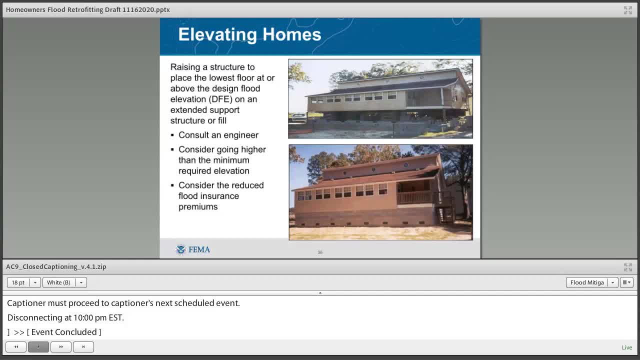 If you were to consider elevating your home, this is raising the structure above, uh, the lowest floor, so your main living area um to or above uh sort of the base flood elevation plus your freeboard or what it may be in some areas. 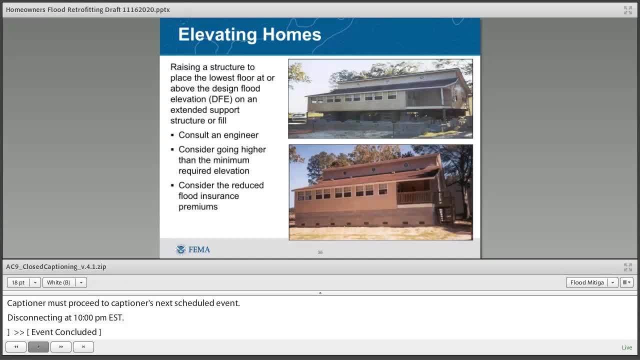 the design flood elevation um on either, you know, columns or maybe sometimes fill, but usually this is columns or an elevated foundation, like we're showing here in the picture. The top picture is a house in eastern North Carolina during the elevation process. 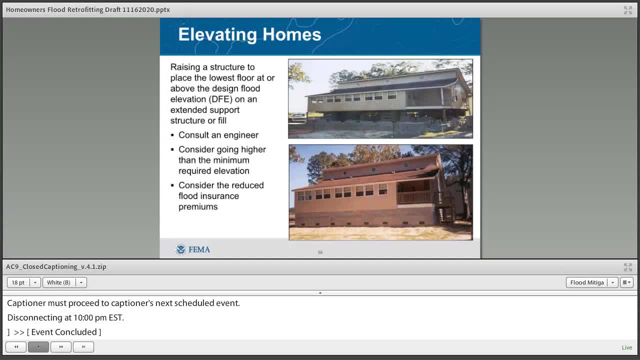 and then the bottom picture is once that that project was completed. Please, please, please, consult an engineer. Don't just use a contractor, but consult an engineer. Uh, we have a lot of buildings, uh in Louisiana that that are on, uh, what we call slab on grade. 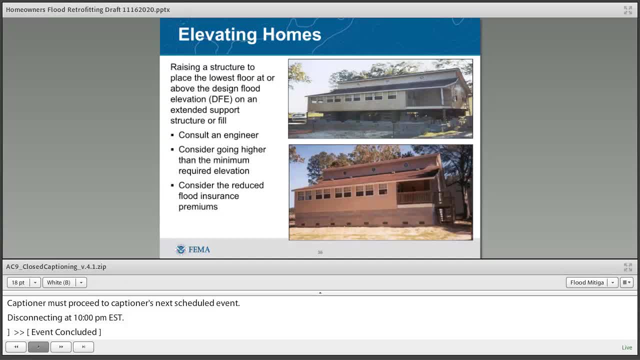 so they're on concrete slabs and I'm gonna show you in a minute why this is so, so important that you consult an engineer. but I would say, regardless of what you're doing, please consult an engineer. This is too much money involved. 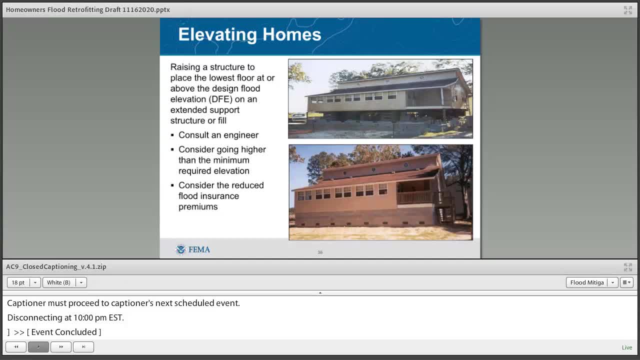 for you not to to get one Uh, consider going higher than what the minimum uh elevation is required. so if the minimum requirement is base flood elevation plus one foot, consider going to base flood elevation plus two foot. It's gonna give you a good bit of risk reduction. 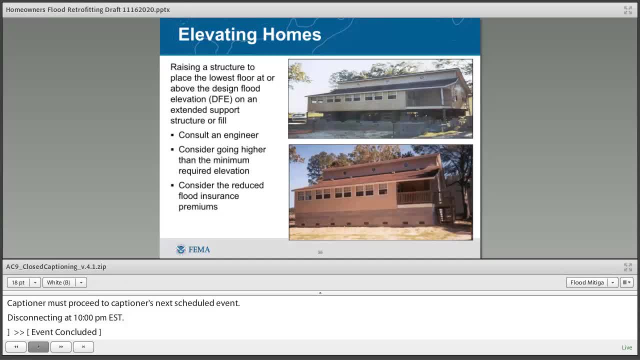 There's all sorts of things that you may consider. Maybe you do have, uh, ductwork under your building and that sort of thing, and maybe you can get that ductwork as high as possible, so that's not gonna be a replacement issue for you. 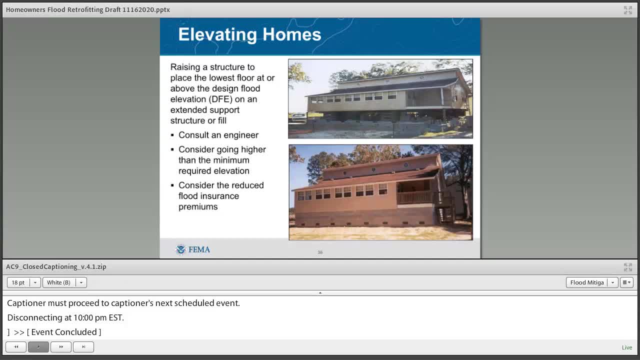 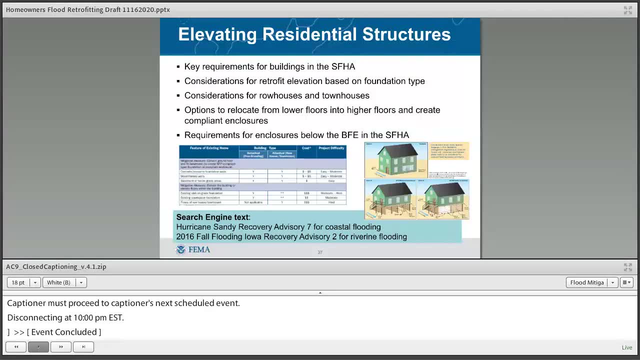 as well as having your reduced flood insurance premiums by going above that minimum elevation required. Uh, we have some guidance on that. we did a Hurricane Sandy Recovery Advisory 7, that's kind of an overview of elevation, and we also did one for the 2016 Iowa floods too. 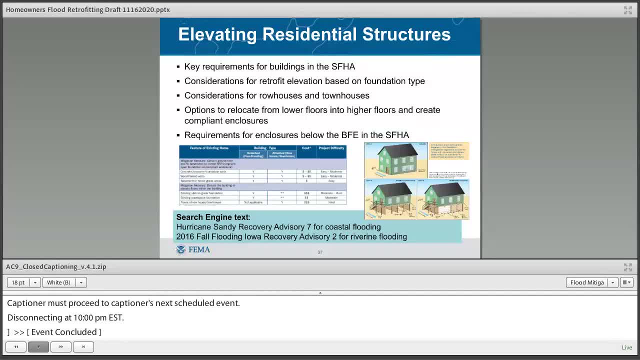 that's Recovery Advisory 2. Uh, one was coastal, one is riverine flooding, um, so those are both helpful. It talks about what those requirements are, uh, what kind of retrofits you can look at um, if you're talking about townhouses, row houses. 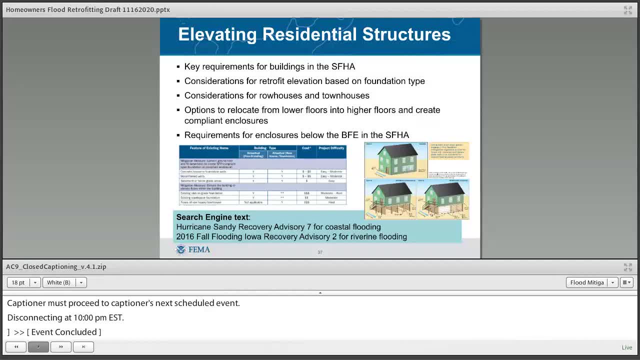 that sort of thing, uh, what the options are for that? um, the other thing that it is going to talk about is enclosures. so what do you do about that area below the base flood elevation? um, as well as sort of changing. 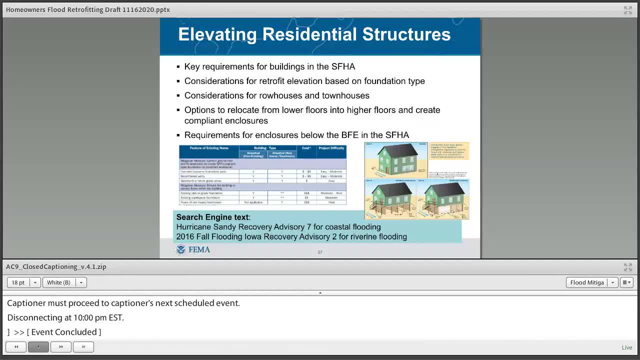 uh, maybe how you've kind of set up the house period, and I'm gonna talk about this just briefly. You've got this diagram that's sort of in the lower right-hand corner and this is um an area where you have a house. 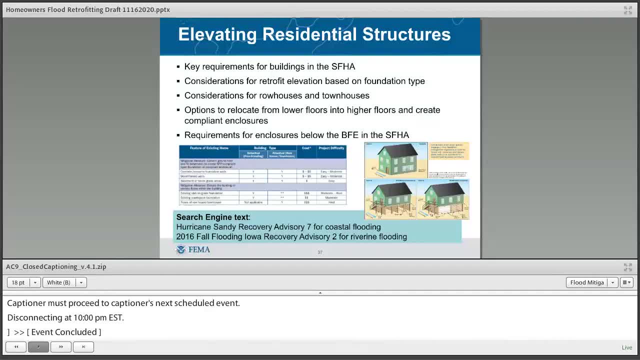 that um was a two-story house, or two-and-a-half-story house, uh, and they abandoned the lowest floor. so they abandoned the first floor, moved out the kitchen and messed the living area into that second floor, uh, and then they've got some. 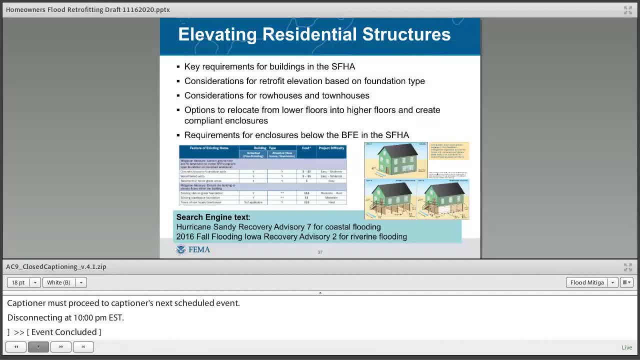 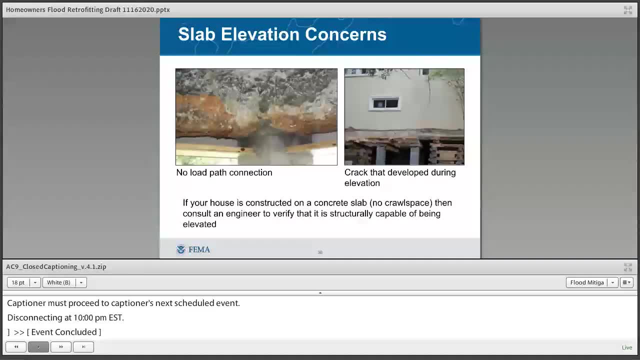 uh breakaway walls and a what we would call a shear wall system below that so that the water can kind of run through that and that system is covered in this. Um, slab elevations, so slab-on-grade uh elevations. 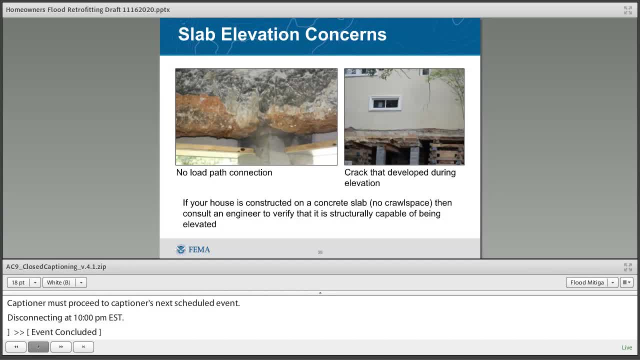 This is where we uh have a house that is constructed, uh, basically, on what we would call a slab-on-grade or slab on the ground. Uh, in those situations, we do see these houses lifted. Uh, when these houses are lifted, 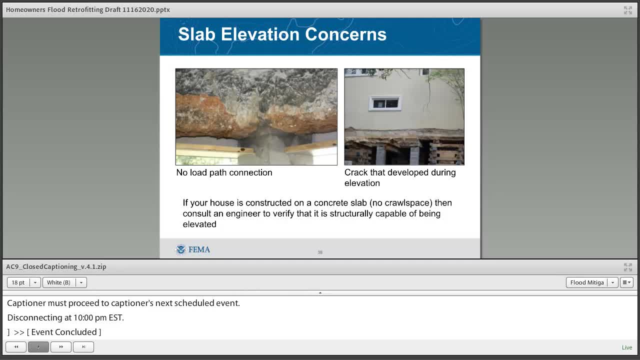 we see um poor load path connections often, so the connection between the columns for that foundation and the slab are often insufficient so that if the house gets pushed sideways by a high wind um that it could get knocked off the foundation. 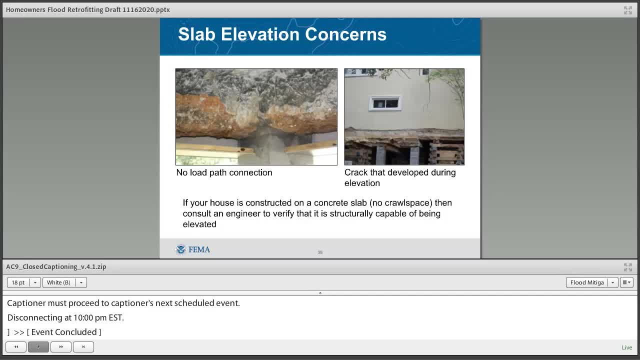 It's not just a matter of how much the house weighs, but also these connections that are important. We also see some houses that are, uh, not elevated correctly, so we see cracks. If you look at the picture on the right, you'll see a crack moving from that top window. 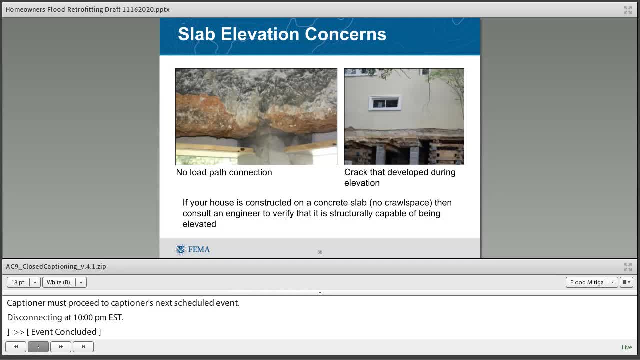 down the the building and- and these are often really difficult to fix because often this crack extends into that slab and that can be a real structural issue. If your house is constructed on a concrete slab, there's no crawl space or anything. 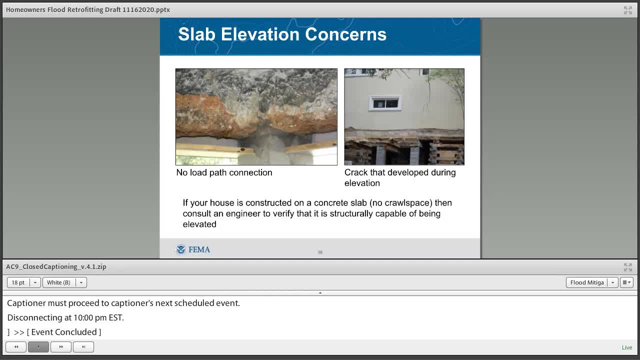 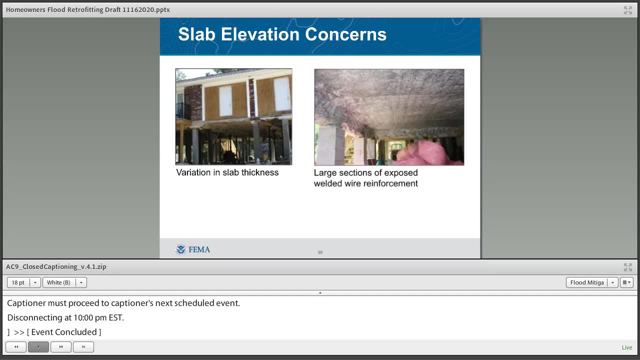 please, please, please, consult, consult an engineer to verify that that house is structurally capable of being elevated. Some more pictures of the issues with this. We see variability in uh slab thickness. The picture on the left uh is a house where the slab actually cracked. 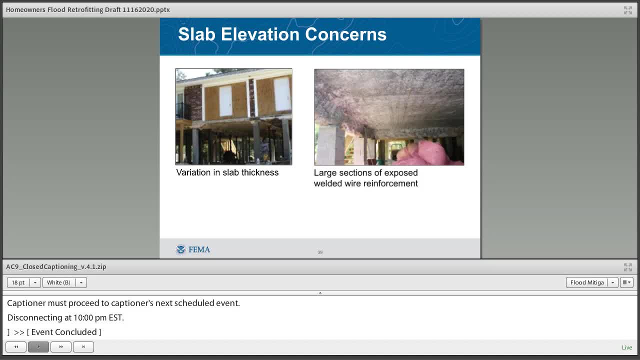 uh, and then the contractor just put a plate over, uh, that crack at the end, but that crack extends all the way through the slab and you could end up with uh that, that slab failing, um, and major structural issues with the house. 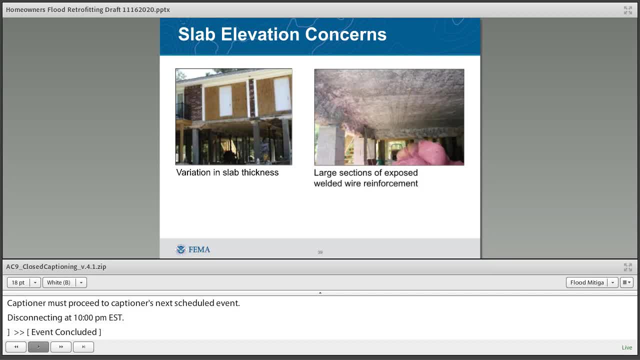 and and potentially hurting the occupants. Uh, the other thing that we see is often the only reinforcement in these slabs is for temperature um and humidity. so this is. you can see in this picture there's some on the right. 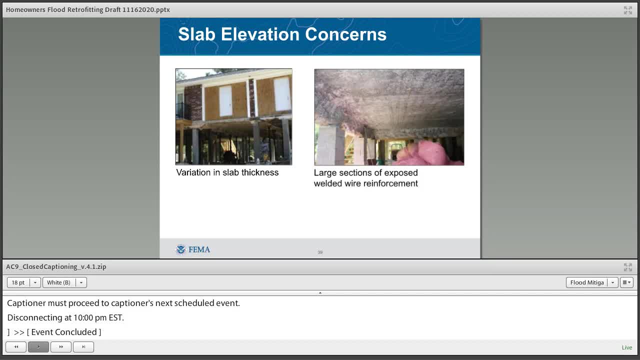 you can see some pieces of of wire fabric. You can see kind of a grid on this slab below it and that's the welded wire fabric. that's only for sort of minimal expansion and contraction in the slab. That's the only reinforcement. 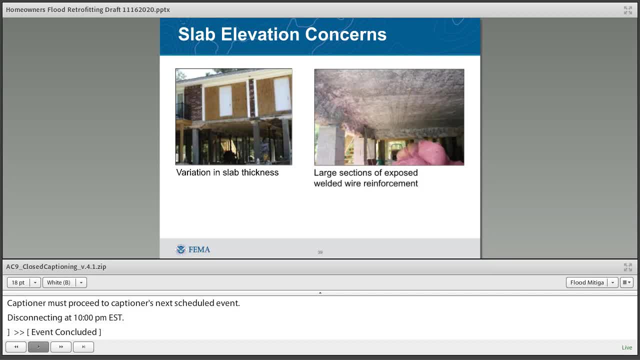 and it was pushed all the way to the bottom of the slab, which means it's not providing any sort of reinforcement. so if the slab is not designed with actual engineered reinforcing in the slab, that is for uh making it a structural slab. 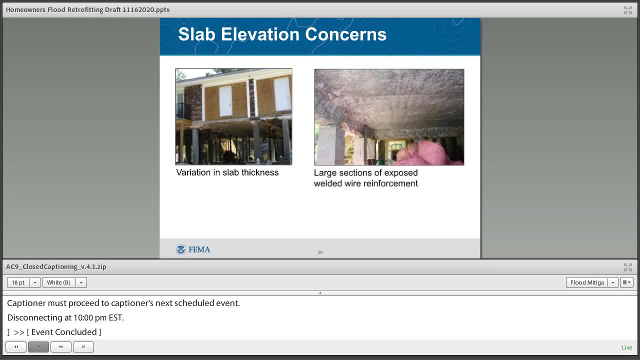 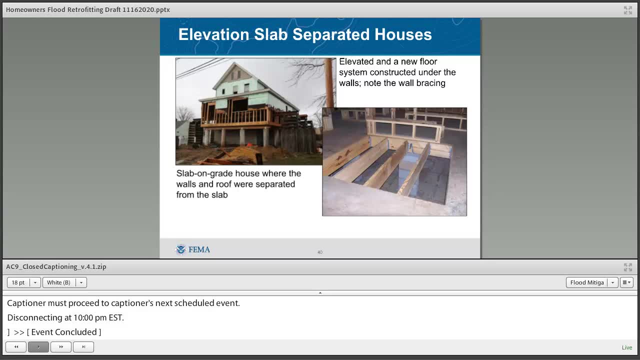 as engineers would call it. if that's not the case, you should not be elevating it, because it's extremely, extremely dangerous. Uh, if you cannot do that, we uh recommend: uh, if you're on a slab on grade. 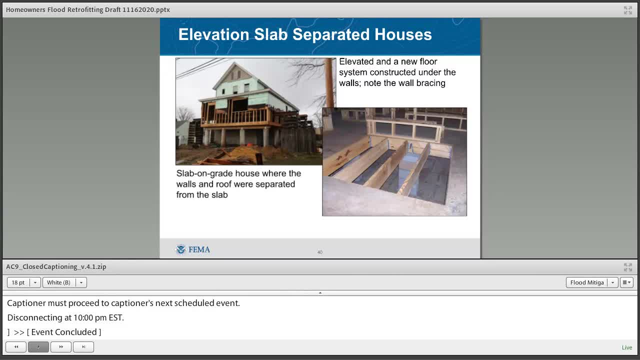 it can't be elevated as a slab. We would recommend a slab-separated house. Uh, this, the house on the right, is sort of- uh, a house in progress that's being elevated. You'll see the picture on the right. Um, this is what they're going to do. 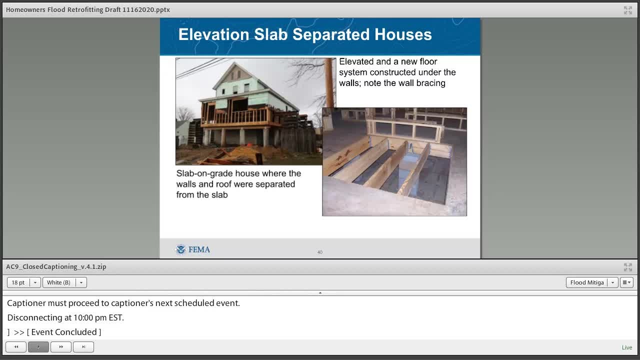 They're going to lift the walls and the roof system and then rebuild a wood-frame floor system, so leaving the original slab on the ground, building new columns above that slab and then, uh, supporting a wood-frame floor system. so you'd move from a slab on grade. 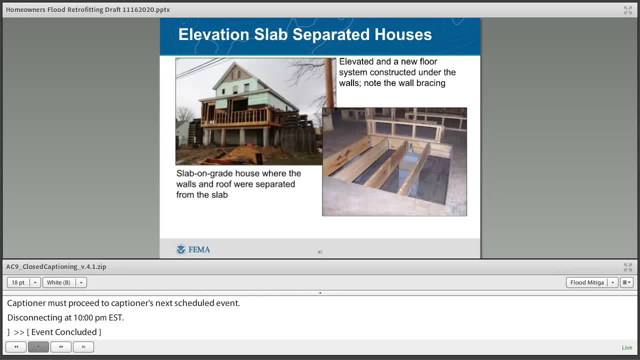 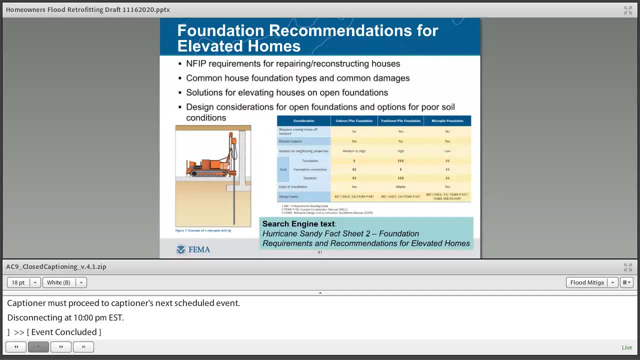 to a wood-frame floor system and this is really the better option for you from a structural capacity standpoint. Um, we do have some Hurricane Sandy fact sheet uh two. That's uh going to give you foundation recommendations If you have any uh issues. 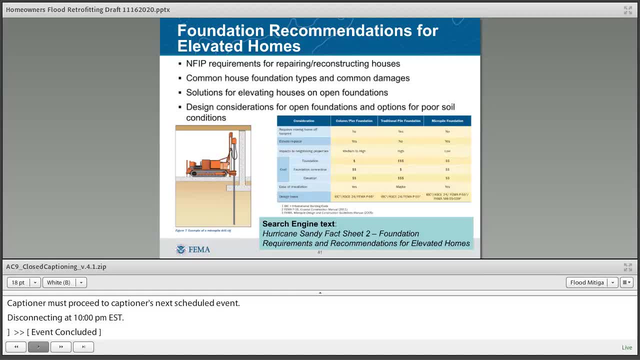 and need some additional uh, foundation support. uh then that's. This gives you some ideas on on, basically, ways that you can shore up or improve the foundation of your house, and sort of the cost and the implications, pros and cons and that sort of thing. 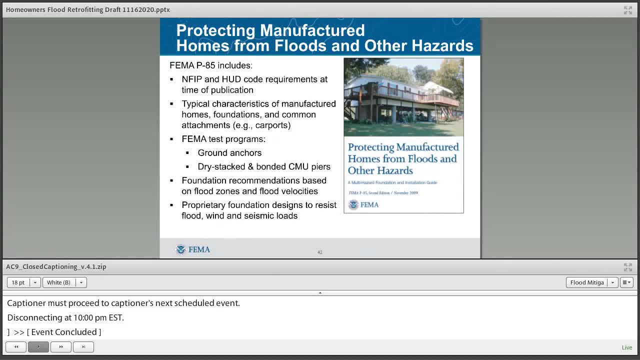 with different types of foundation systems. Um, if you have a manufactured home, I would recommend you look at FEMA P-85.. Um, that's protecting manufactured homes from floods and other hazards. This is, uh going to give you some good guidance. 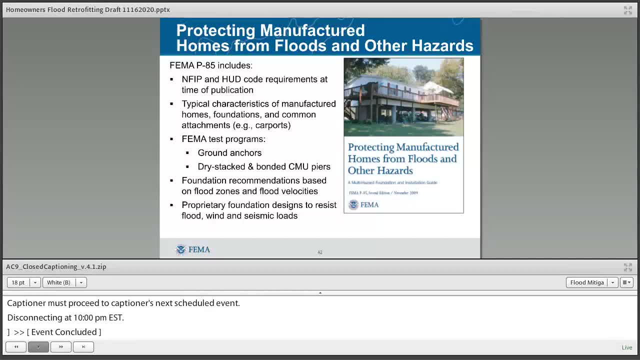 on not only flood protection but also high-wind uh protection and it'll give you some ideas on foundations and there's actually some uh prescriptive plans and that sort of thing for foundations and anchorage systems and that sort of thing for manufactured homes. 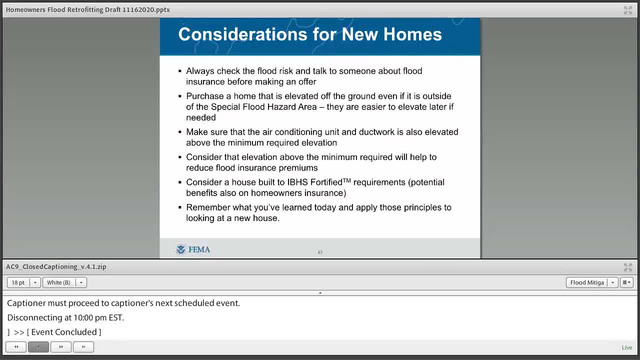 Uh, the last thing I want to talk about is considerations for new homes. Uh, trust uh only yourself with looking at the flood risk. Uh, make sure that you check out the flood risk and talk to somebody about flood insurance before even making an offer on a house. 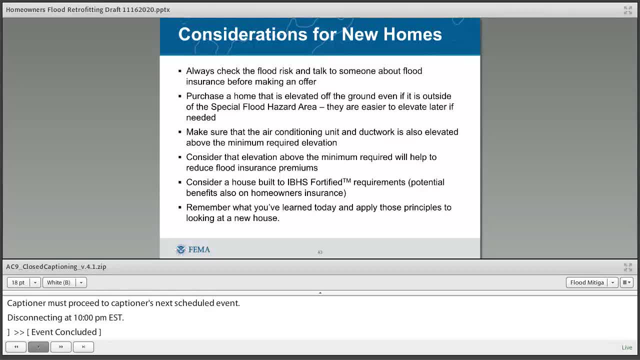 Um, don't find out about the flood risk after you've signed any of the paperwork and and check this out yourself. I can't ex? uh- you know stress this- enough how important this is. Uh, purchase a home that's elevated off the ground. 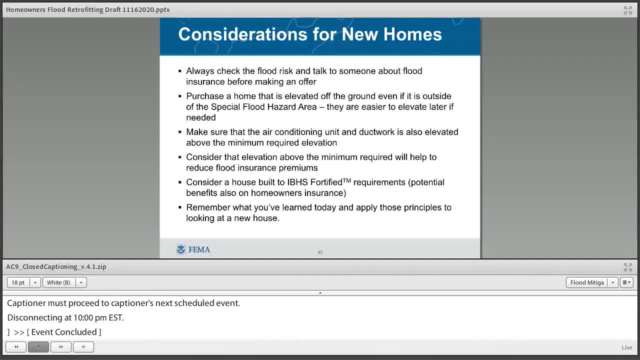 even if it's outside the special flood hazard area. Uh, if the flood hazard area expands over time due to things like subsidence or anything like that, uh, then that can make the house easier to elevate later, if that's needed. Uh, make sure that the air conditioning unit. 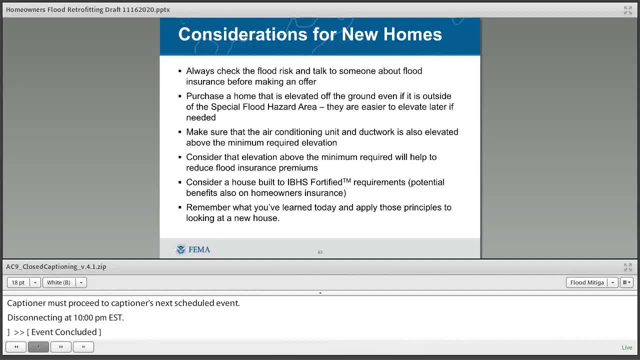 and the ductwork is also elevated above the minimum elevation requirements. Um, consider elevation above the minimum because this can reduce, uh the reduce, your flood insurance premiums. Consider a house that, uh, here's we. we get to the Insurance Institute. 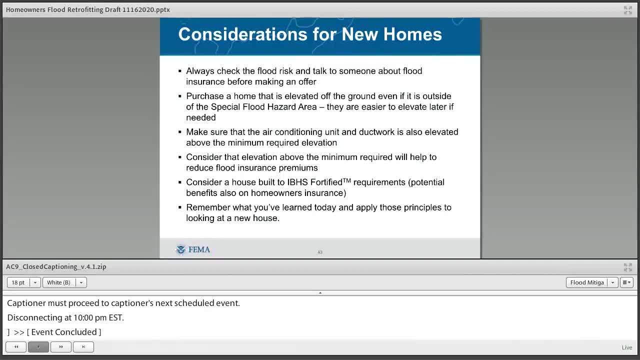 for Business and Home Safety, IBHS, The IBHS fortified system. Uh, there are potential benefits to your homeowner's insurance. See if you can find a house that's constructed to those requirements and that would be really helpful for you. Uh, both from a flood perspective. 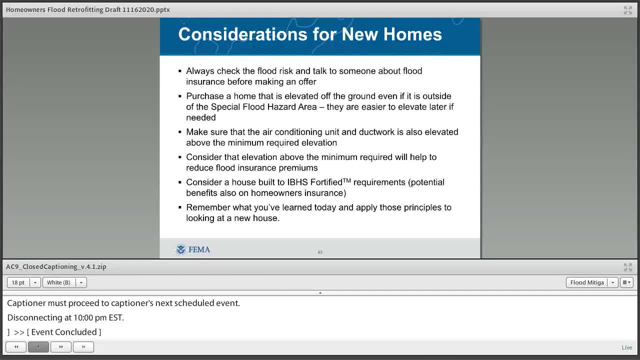 reduced uh flood risk as well as high wind protection. Um and again, there may be benefits uh through your homeowner's insurance policy for that, in addition to the higher elevation which would help you on your flood insurance. Remember what you've learned today. 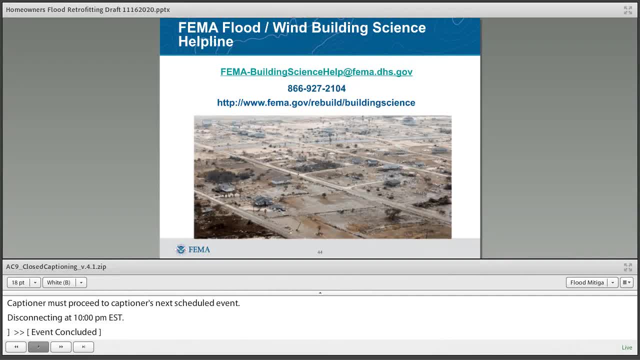 in uh applying those principles to looking at a new house. Uh, the last thing I want to touch on is there is a FEMA Building Science, Flood and Wind Helpline. Uh, you'll see the uh address there. There's an email address there that you can. 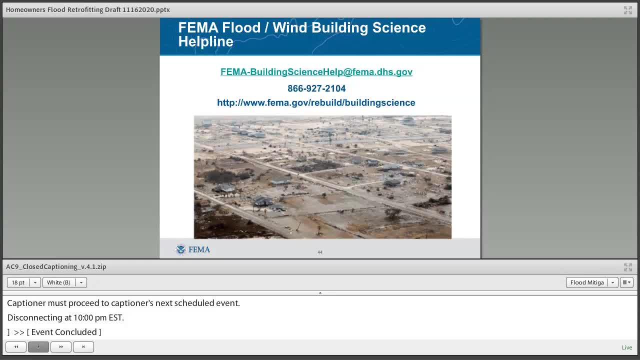 you can contact, Or there's a phone number and you can leave a message. We'll get back to you within a few days to answer your questions. We can't answer questions specific to issues- uh, issues with your specific house- but we can. 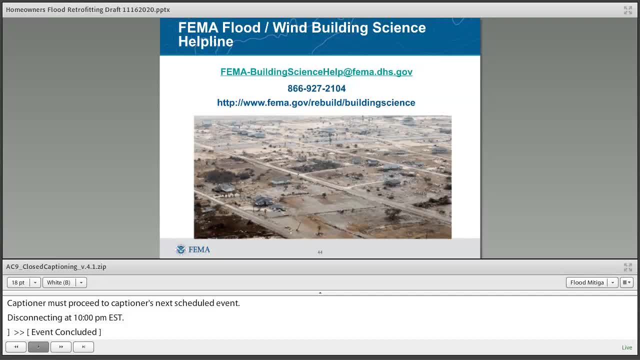 we can answer generic sort of building science questions about what the policy is, what the recommendations are, where to find information and that sort of thing. So, uh, if that's helpful for you, um, we can provide that And this concludes, uh, my discussion. 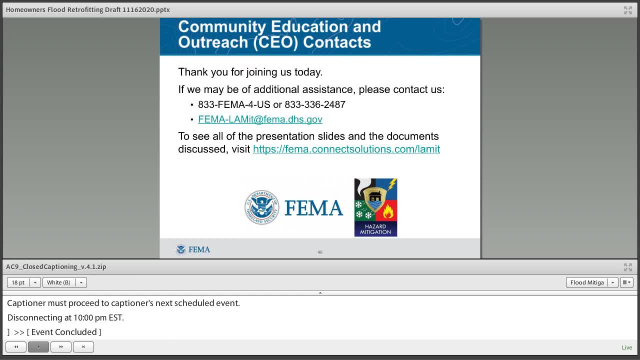 Thank you, Adam. That was great information that you've given us. I want to thank everyone joining us today. We appreciate your participation. We want to send the information to you today, but we also would like for you to contact us if you have any additional information. 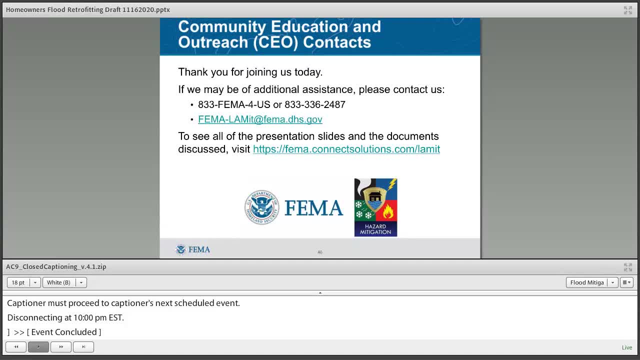 at our FEMA uh mitigations um e- um email address at FEMA-LAMIT at femadhsgov, or you, or or you can see our slides and this presentation at our FEMA connect solutions dot com. Thank you again, Adam. Really appreciate your time.